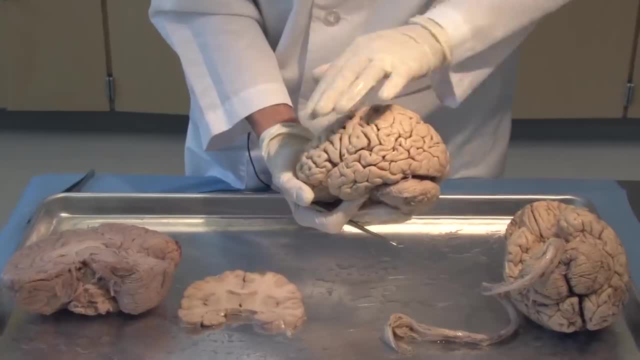 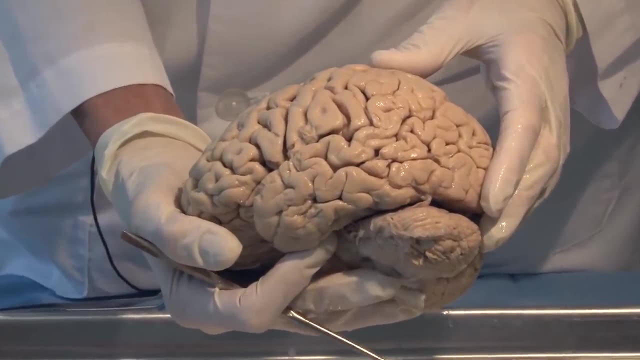 brain. Now let's look at the surface of the brain. We've removed the coverings, the leptomeninges, the pia and the arachnoid, and I want to just show you the different lobes of the brain as an introduction. 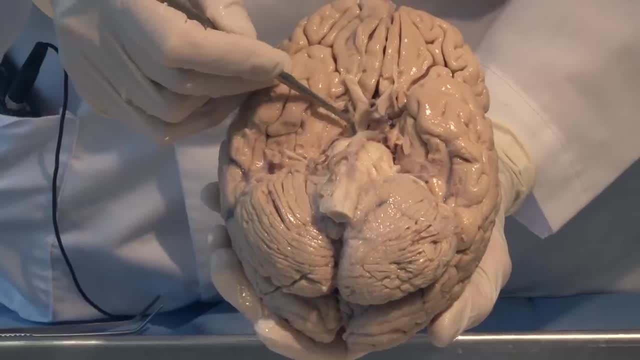 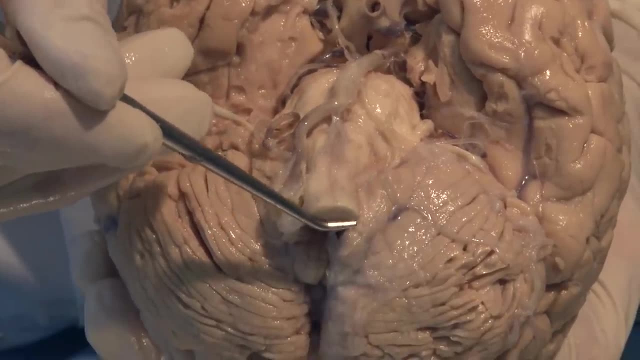 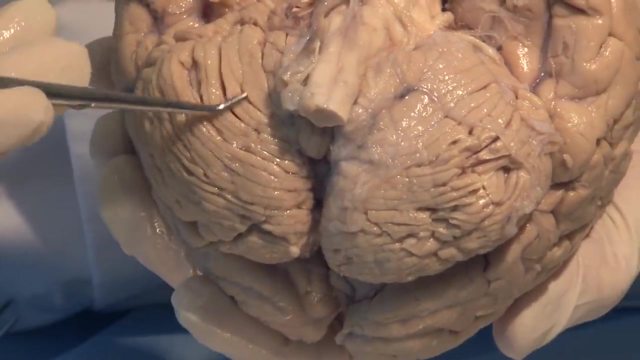 You can see the brain stem. The brain stem extends from this region, where my probe is a little bit difficult to see, down all the way here to where the spinal cord was attached. In addition, you can see the cerebellum involved with coordinated motor control, as well as. 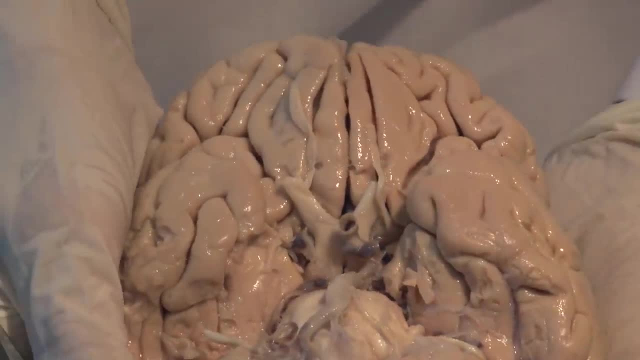 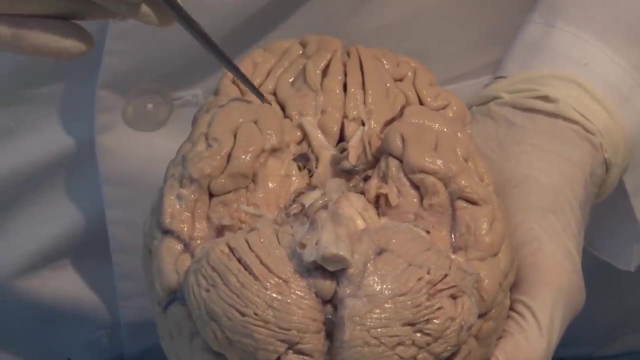 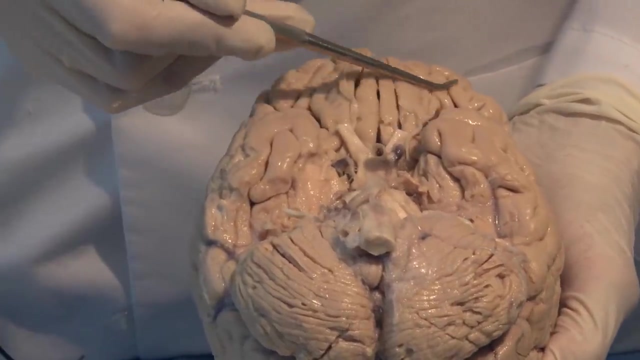 the surface of the cerebral cortex. This is the ventral surface of the brain And the most prominent feature here is the temporal lobe, which I am outlining. Here is the temporal lobe on the other side, And in front of it is the undersurface of the frontal lobe. 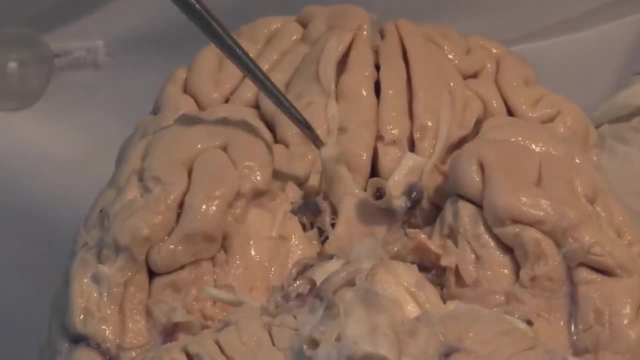 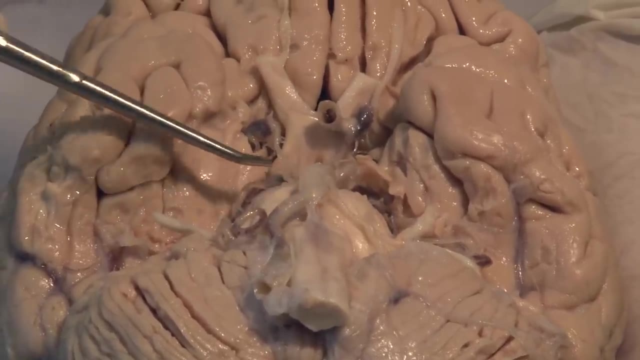 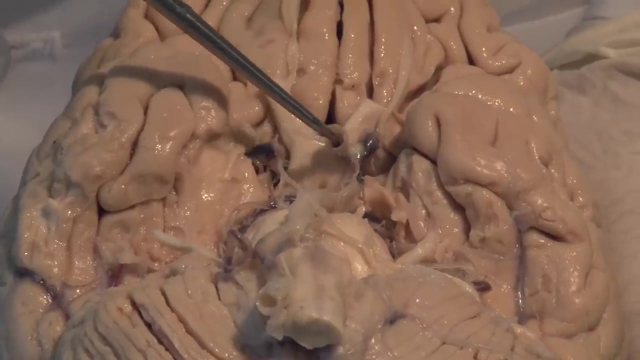 Cranial nerves are attached, such as the visual optic nerve and the sensory nerve from the face, the trigeminal nerve and blood vessels such as this large basilar artery. These are running on the surface Or you can even see the large internal carotid artery. 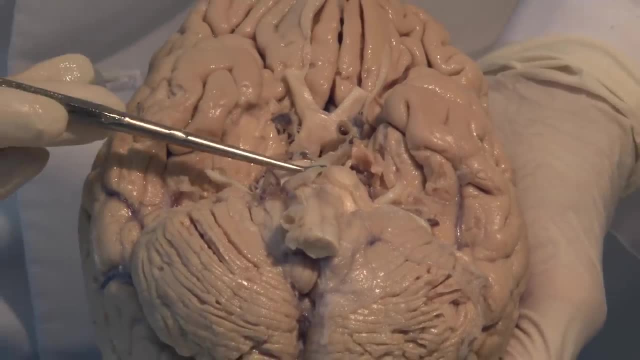 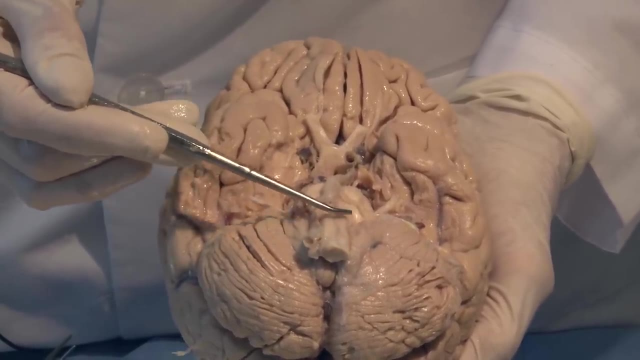 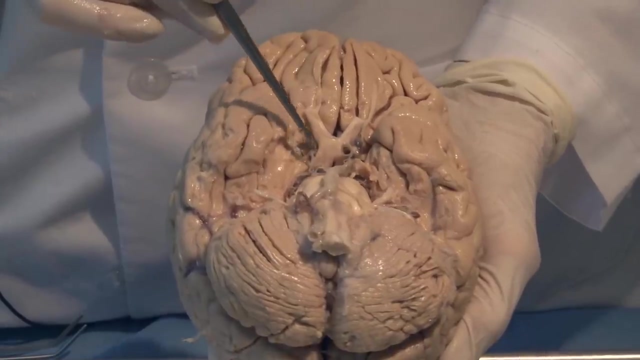 We will come back and look at the nerves and the arteries and the other connections in greater detail, But I just want to introduce you to the region of the medulla, the pons and the midbrain, And together they make up the brain stem. 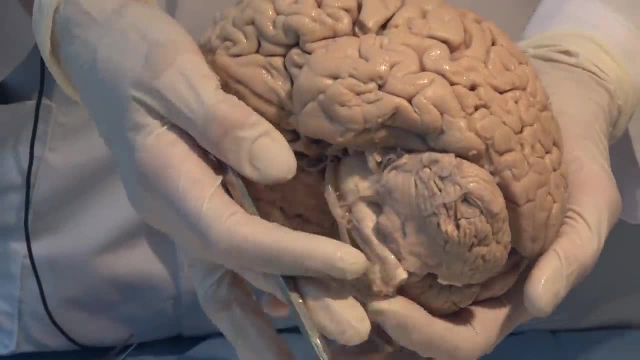 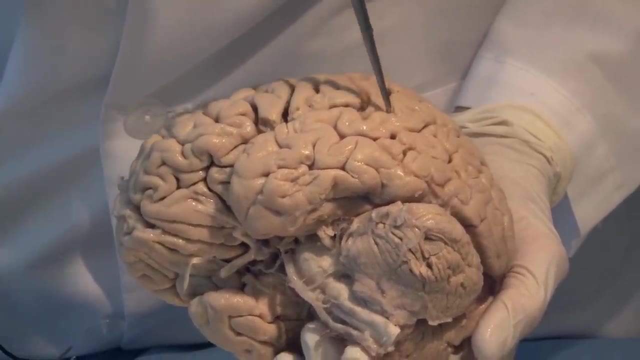 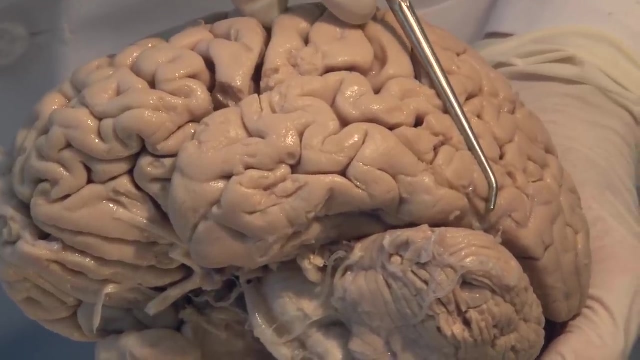 Let's look at the surface now of the brain And look at the different lobes. You already saw the inferior surface of the temporal lobe coming back to here, And we just kind of arbitrarily draw a line and say that this is approximately the end of the temporal lobe. 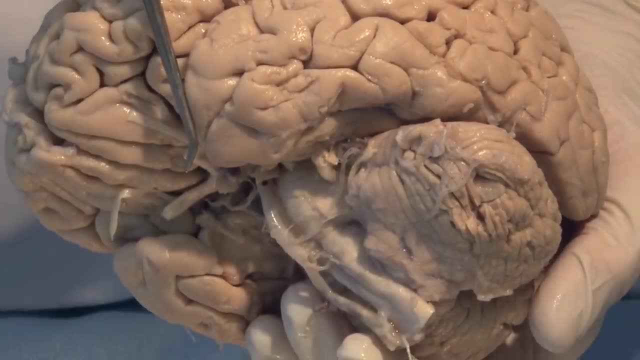 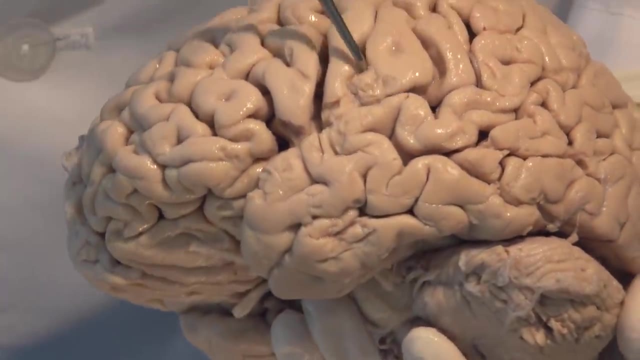 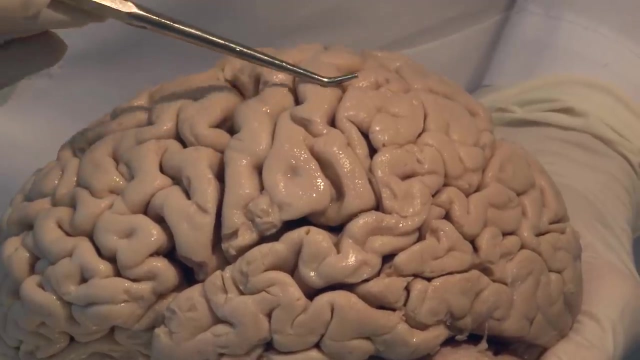 posteriorly and the tip of the temporal lobe anteriorly. And then we look for a sulcus on the surface of the brain. Sulci are these grooves And the surface structures that are coiled are the gyri. So we have sulci and we have gyri. 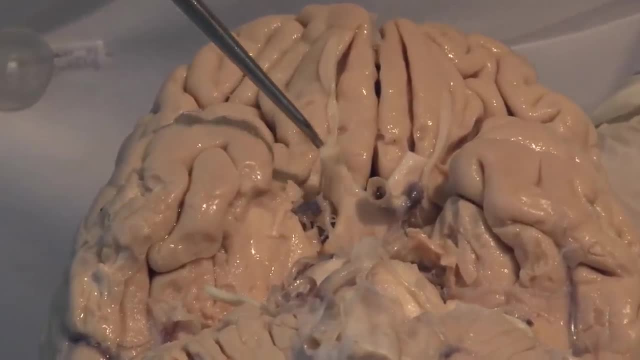 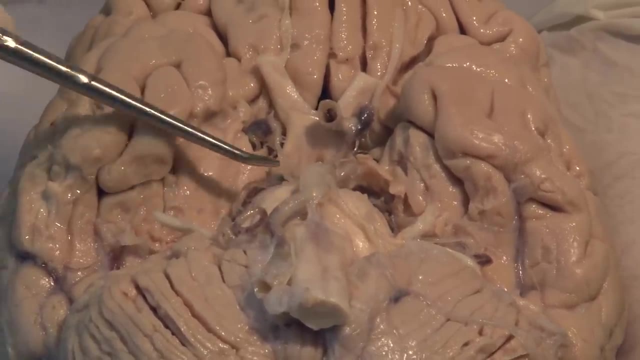 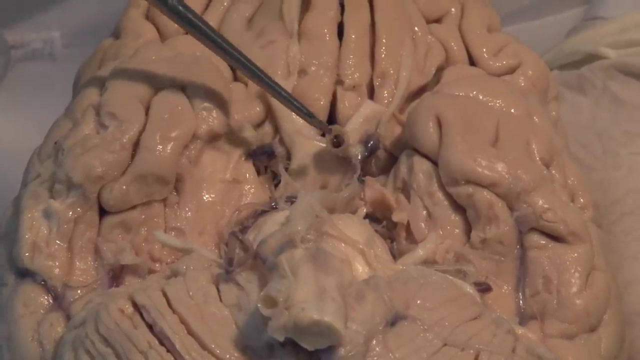 Cranial nerves are attached, such as the visual optic nerve and the sensory nerve. from the face, the trigeminal nerve And blood vessels, such as this large basilar artery, are running on the surface, Or you can even see the large internal carotid artery. 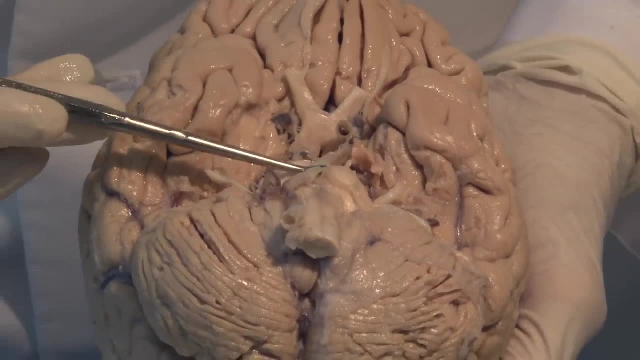 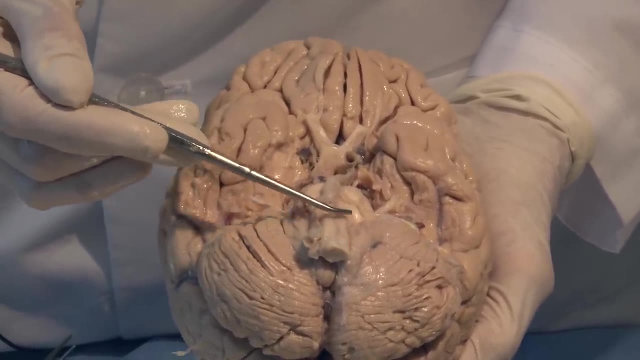 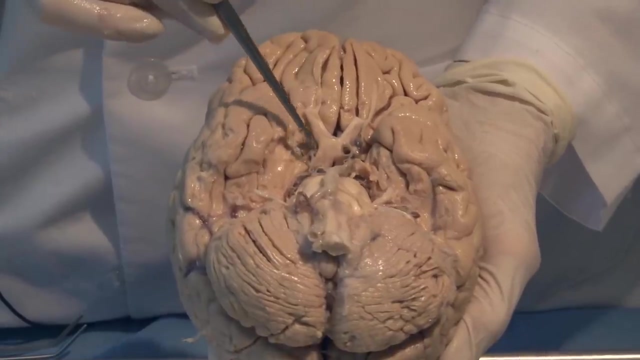 We will come back and look at the nerves and the arteries and the other connections in greater detail, But I just want to introduce you to the region of the medulla, the pons and the midbrain, And together they make up the brain stem. 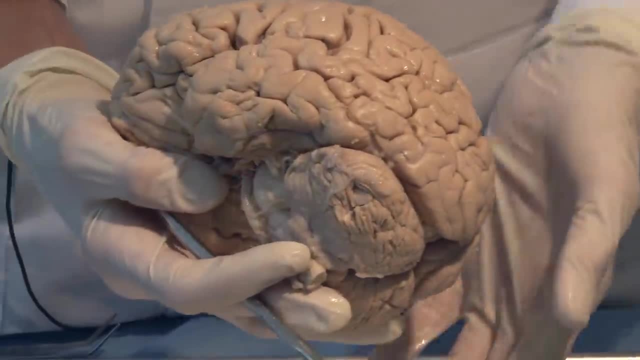 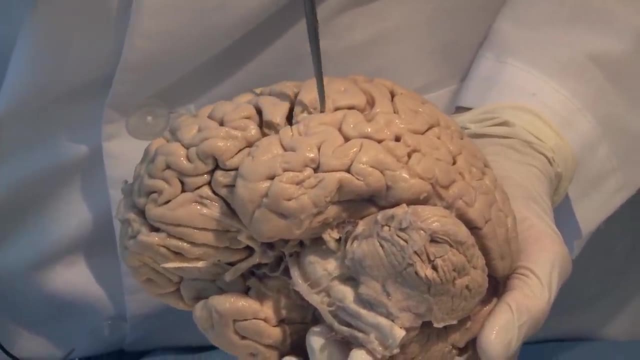 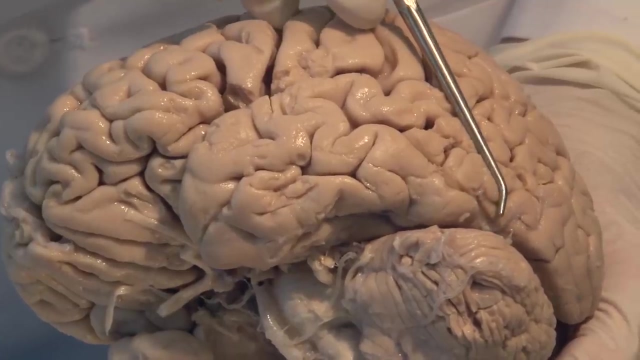 Let's look at the surface now of the brain and look at the different lobes. You already saw the inferior surface of the temporal lobe coming back to here, And we just kind of arbitrarily draw a line and say that this is approximately the end. 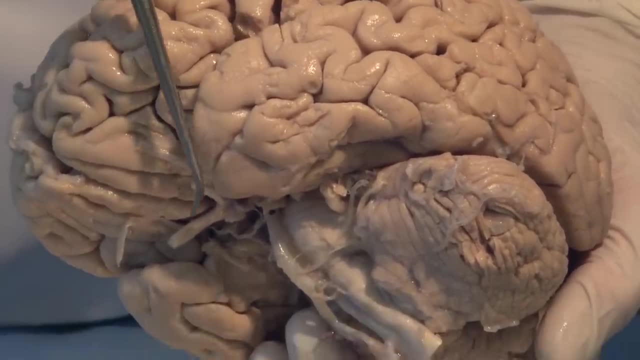 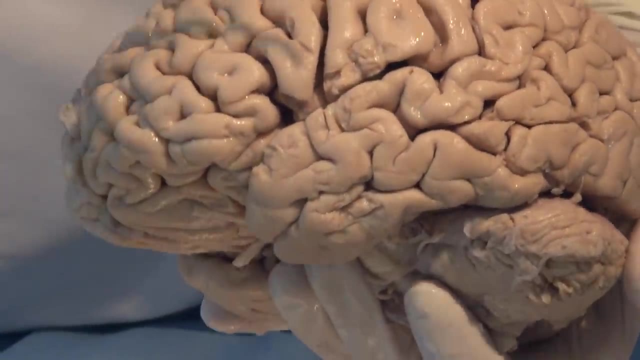 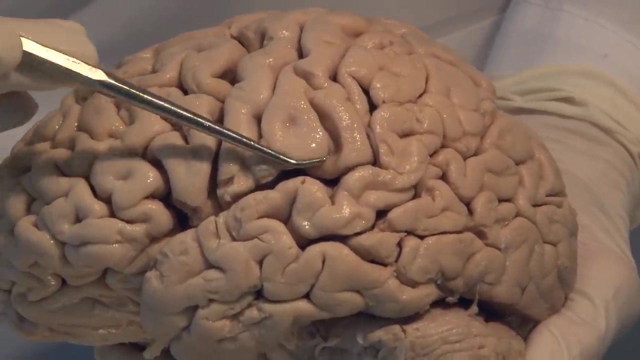 of the temporal lobe posteriorly and the tip of the temporal lobe anteriorly, And then we look for a sulcus on the surface of the brain. Sulci are these grooves And the surface structures that are coiled are the gyri. 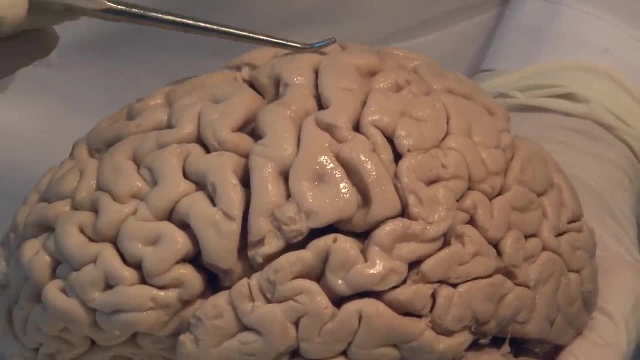 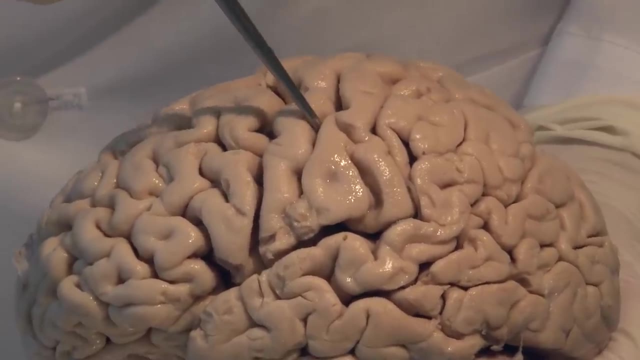 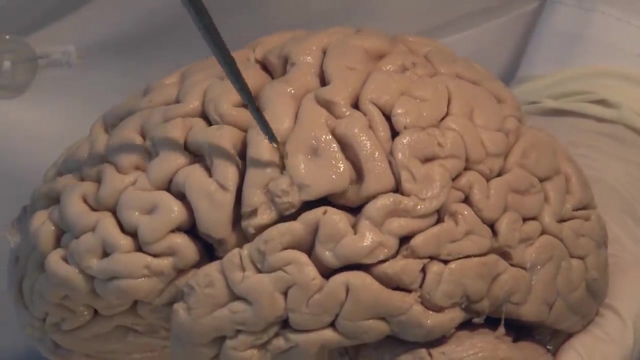 So we have sulci and we have gyri. The gyri have names, but we're not going to learn most of them. However, this major sulcus, the central sulcus, because it runs from the midline all the way down to the lateral fissure separating it from the temporal lobe- 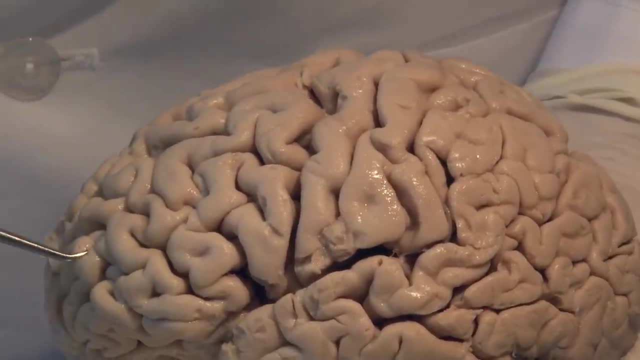 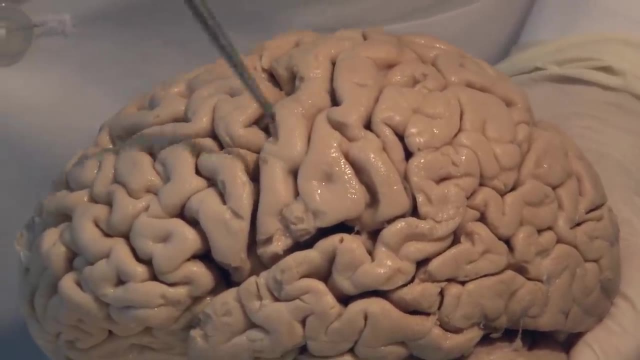 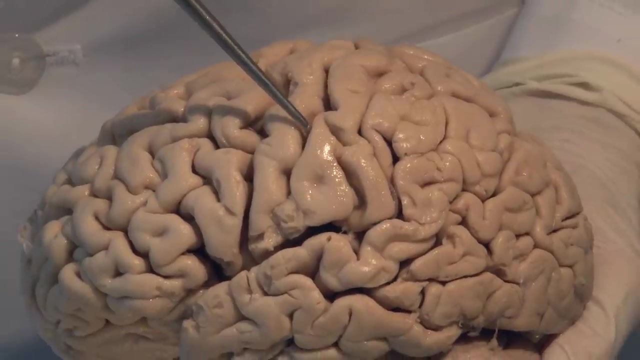 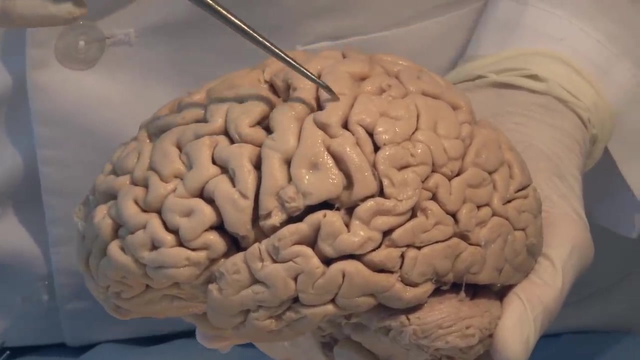 This central sulcus separates frontal lobe in front of it from parietal lobe behind it And, very interestingly, the cortex involved in voluntary movement is in front of the central sulcus And the cortex involved with primary somatic sensation from your body is the gyrus behind the central sulcus. 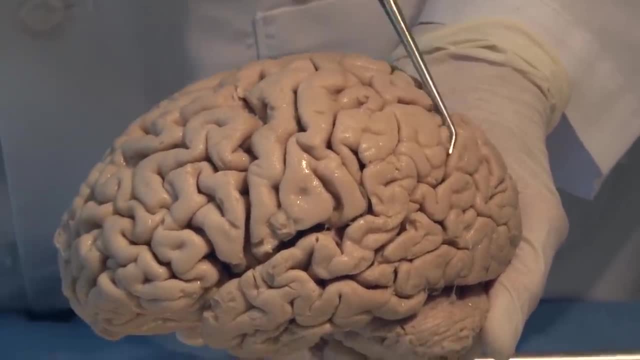 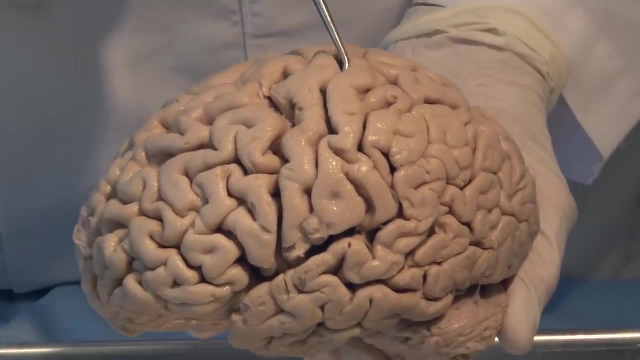 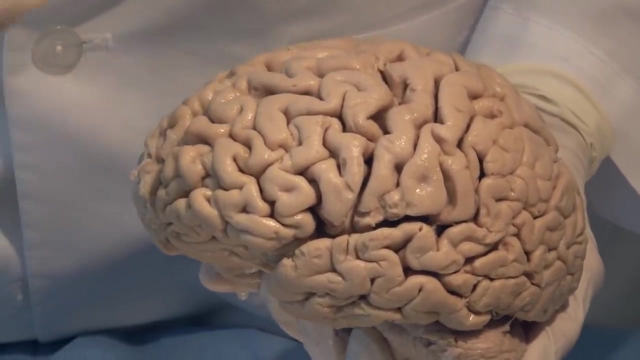 So this is frontal lobe, This is parietal lobe, This is motor cortex in general And this is sensory cortex in general. So we're just getting our bearings. The frontal lobe is further sort of divided And it's hard to see the distinction. 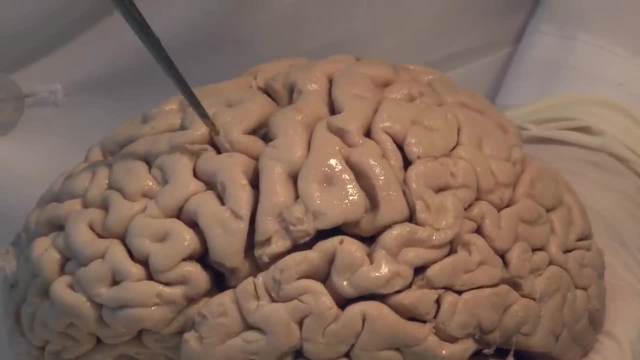 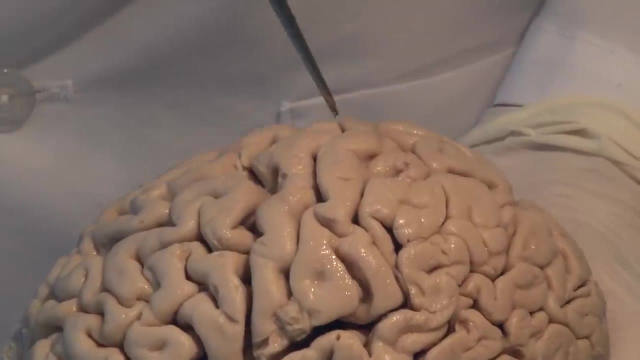 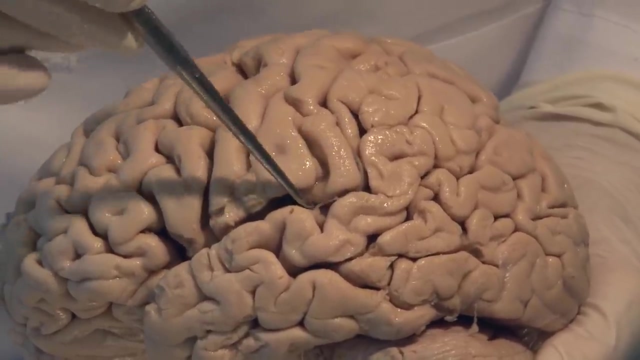 The gyri have names, but we're not going to learn most of them. However, this major sulcus, the central sulcus, because it runs from the midline all the way down to the lateral fissure separating it from the temporal lobe- 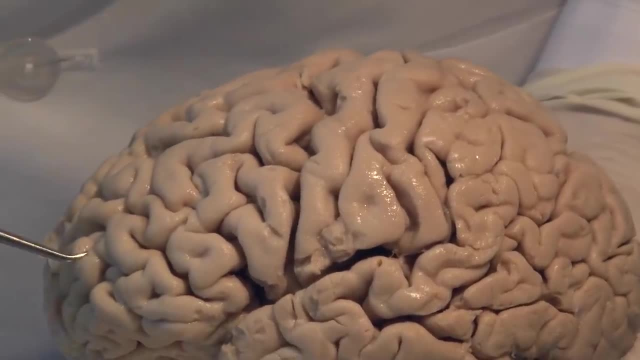 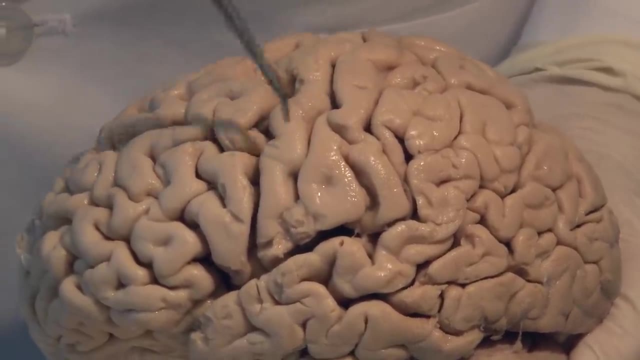 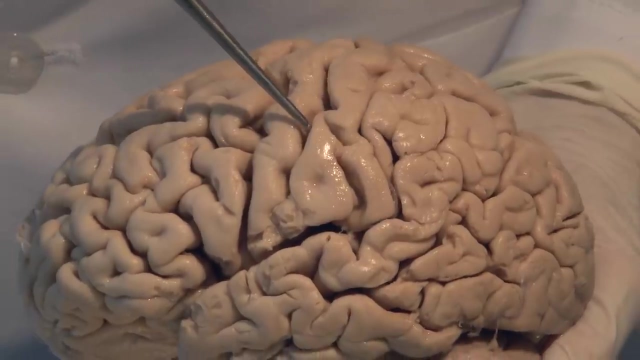 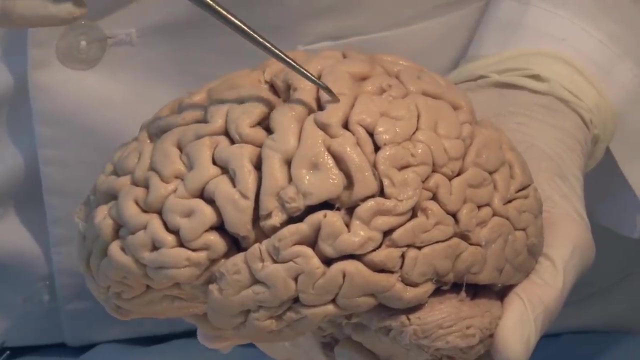 this central sulcus separates frontal lobe in front of it from parietal lobe behind it And, very interestingly, the cortex involved in voluntary movement is in front of the central sulcus And the cortex involved with primary somatic sensation from your body is the gyrus behind the central sulcus. 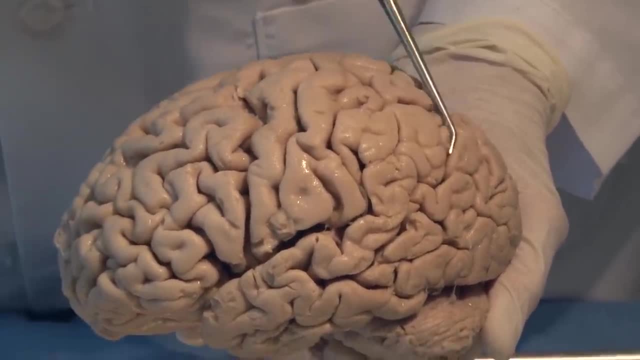 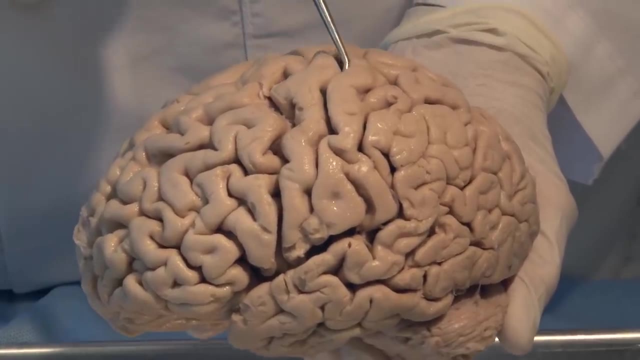 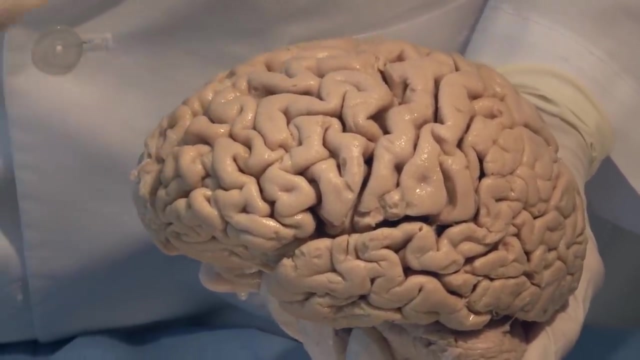 So this is frontal lobe, This is parietal lobe, This is motor cortex in general And this is sensory cortex in general. So we're just getting our bearings. The frontal lobe is further sort of divided And it's hard to see the distinction. 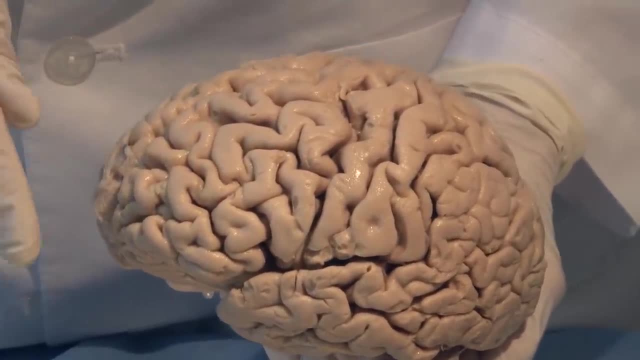 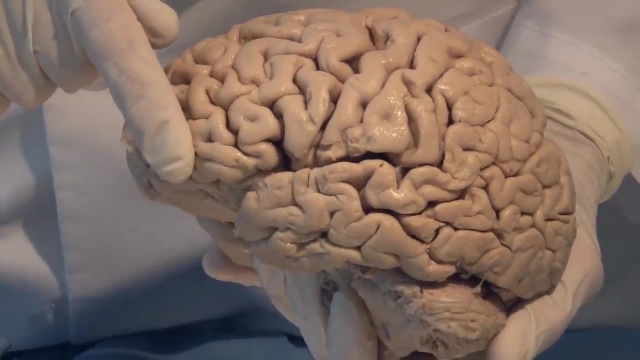 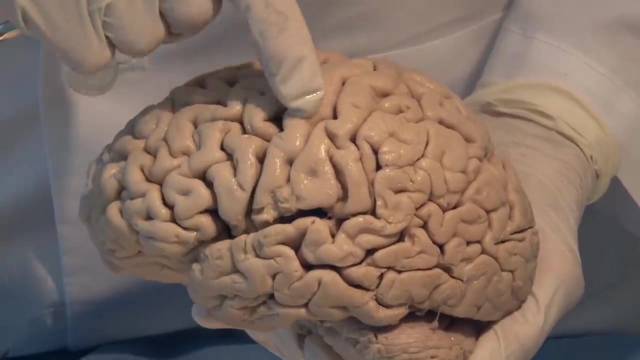 But this band along here is the superior frontal gyrus, Then we have the middle frontal gyrus And the inferior frontal gyrus, The motor cortex in front of this precentral gyrus, as we call it, because it's in front of the central sulcus. 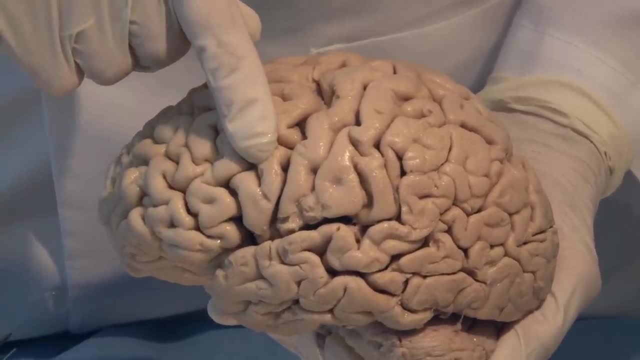 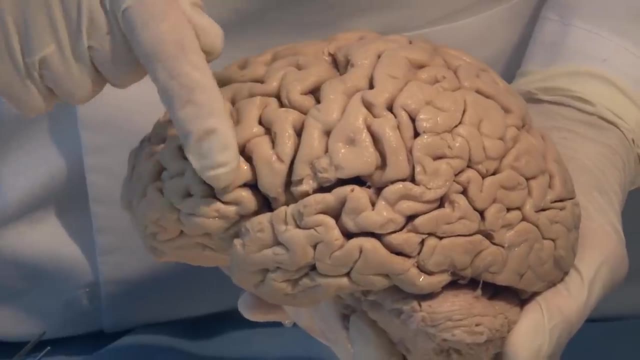 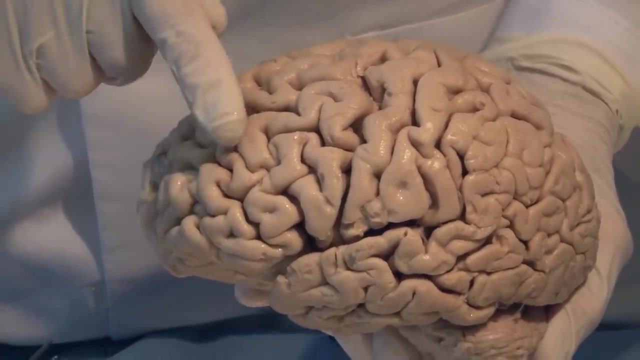 is an area involved in the left hemisphere which we're looking at with the production of speech, And you may have heard of it before: It's called Broca's area. The rest of the frontal lobe is either motor function, planning motor function. 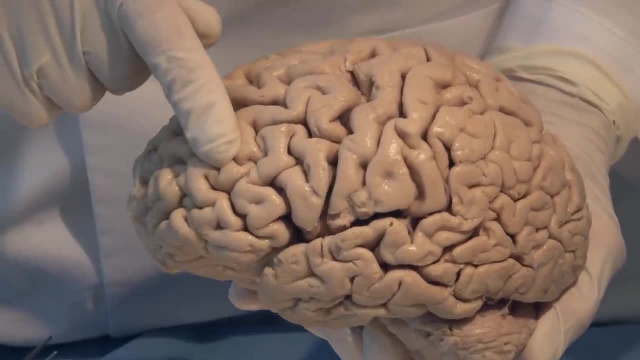 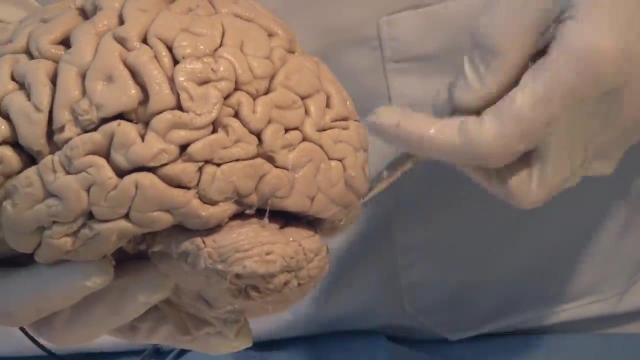 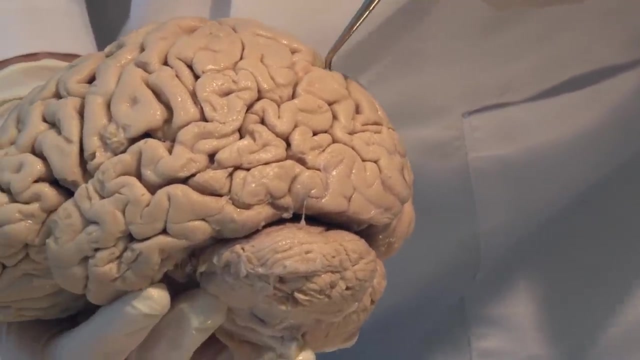 or executive function, such as judgment and planning. Let's look at the parietal lobe now. The parietal lobe is separated from the occipital lobe by an arbitrary line that we draw between the parietal and the occipital regions. these little notches here. 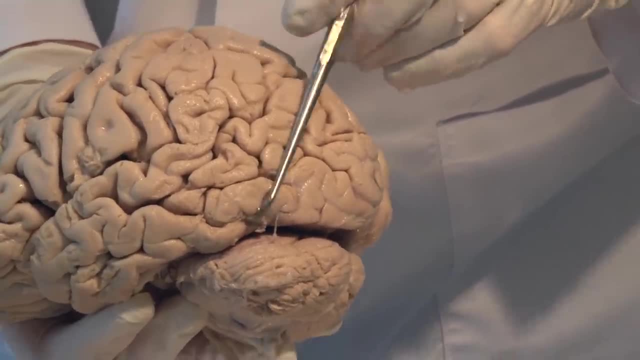 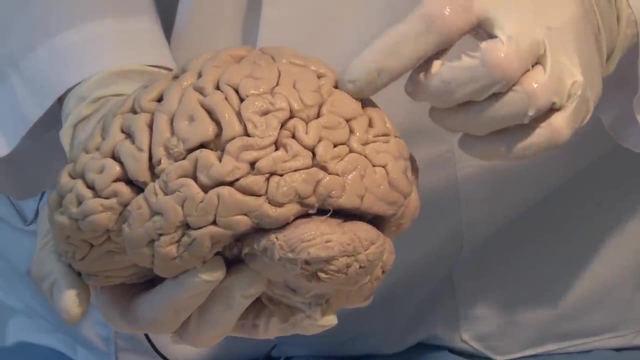 So if I were to display here, I would say that approximately this is the occipital lobe. The occipital lobe is very important in humans because this lobe is involved with visual information processing. It's a wonderful brain that we have. 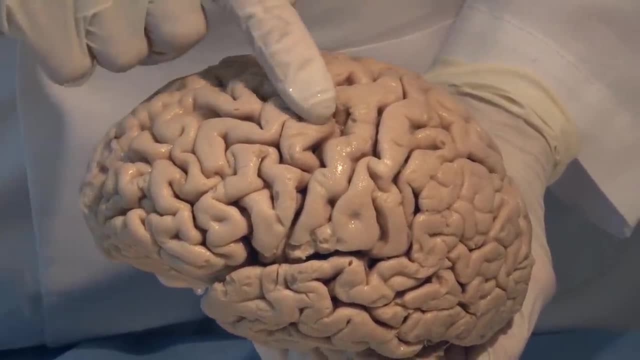 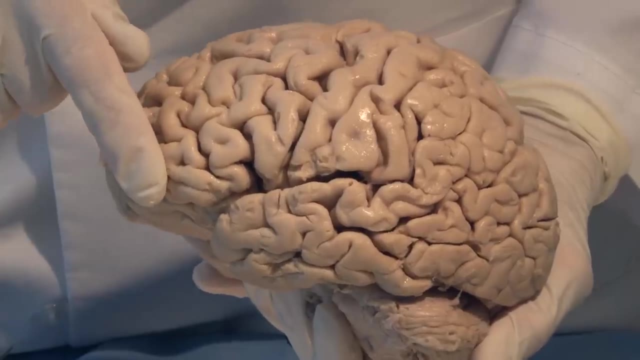 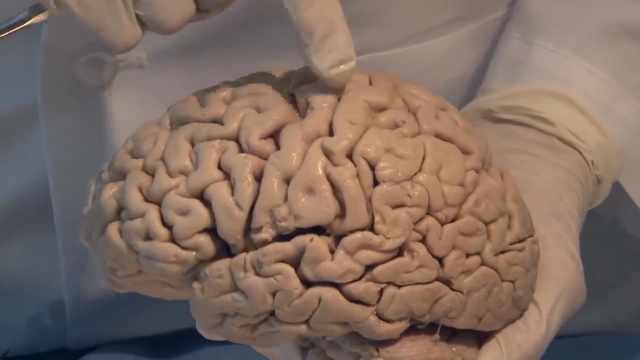 But this band along here is the superior frontal gyrus, Then we have the middle frontal gyrus and the inferior frontal gyrus, The motor cortex in front of this precentral gyrus, as we call it, because it's in front of the central sulcus. 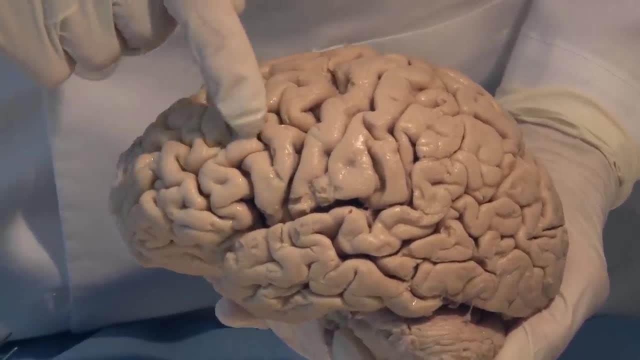 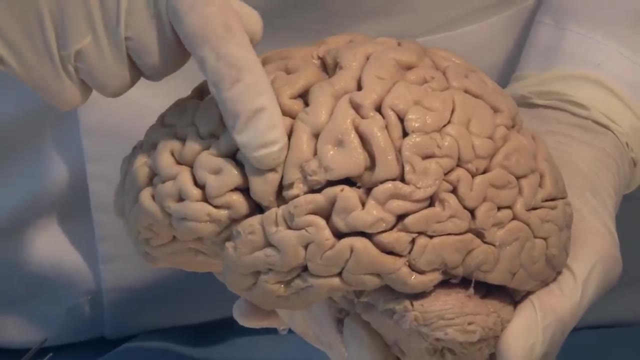 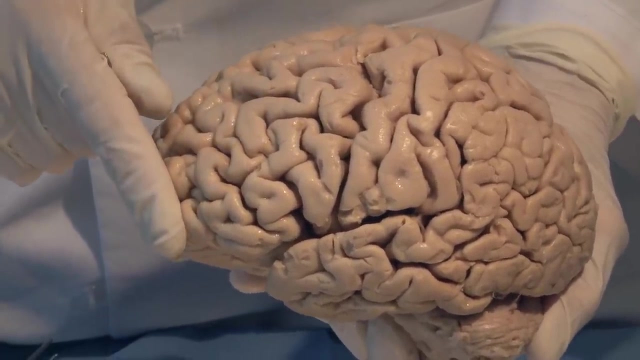 is an area involved in the left hemisphere which we're looking at with the production of speech, And you may have heard of it before: It's called Broca's area. The rest of the frontal lobe is either motor function, planning motor function. 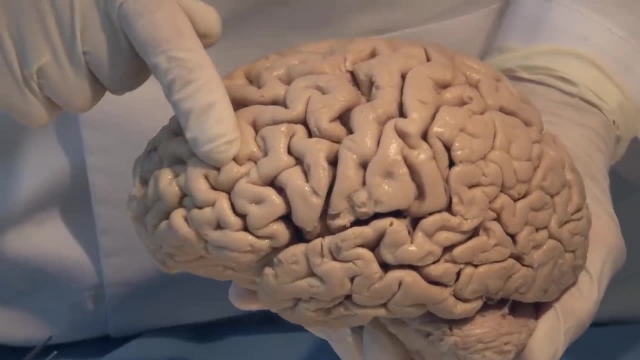 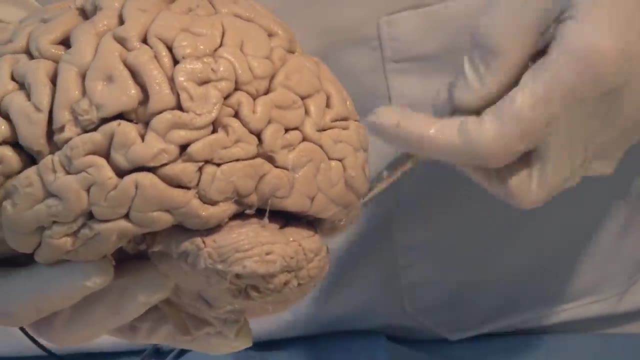 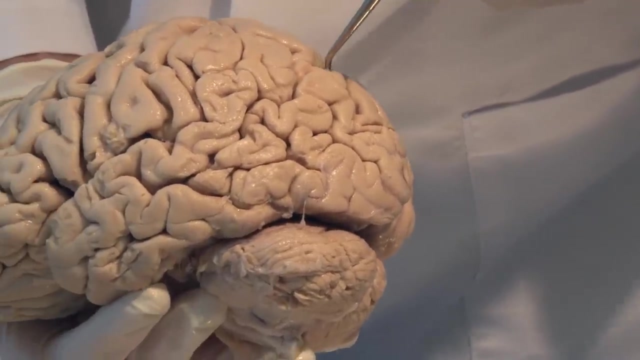 or executive function, such as judgment and planning. Let's look at the parietal lobe now. The parietal lobe is separated from the occipital lobe by an arbitrary line that we draw between the parietal and the occipital regions. these little notches here. 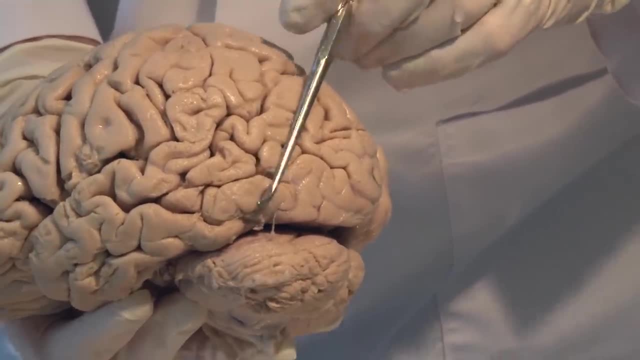 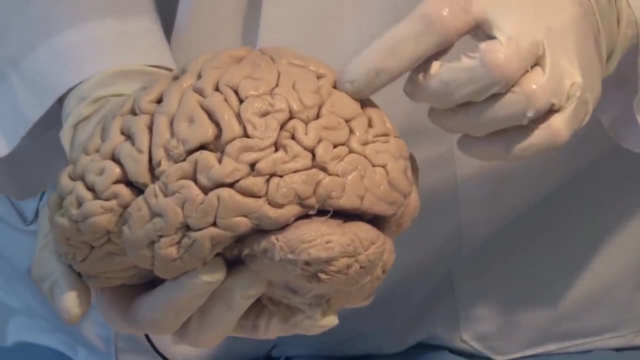 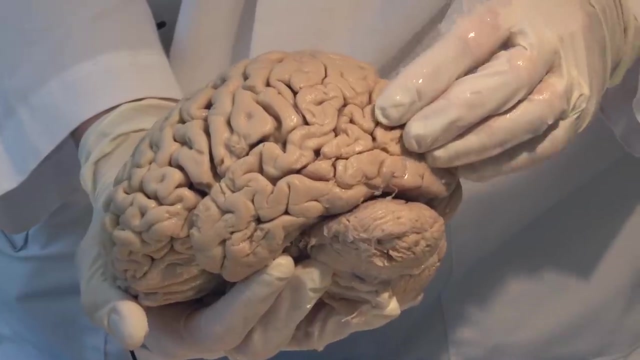 So if I were to display here, I would say that approximately this is the occipital lobe. The occipital lobe is very important in humans because this lobe is involved with visual information processing. It's a wonderful brain that we have and we are very specialized as humans. 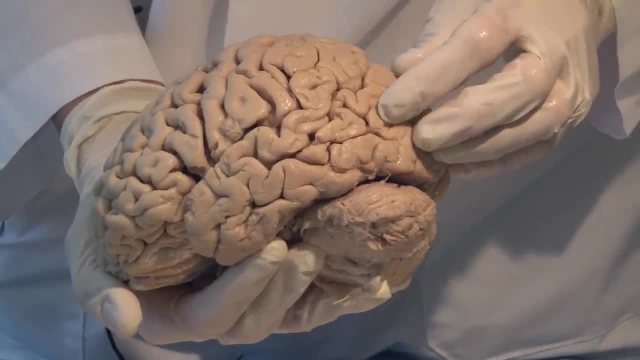 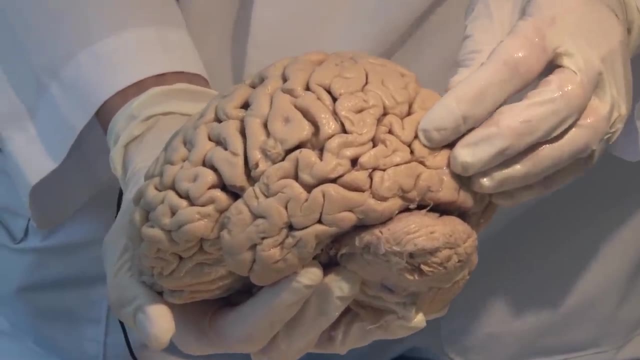 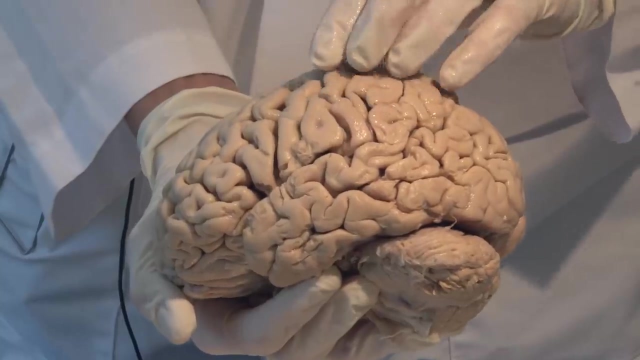 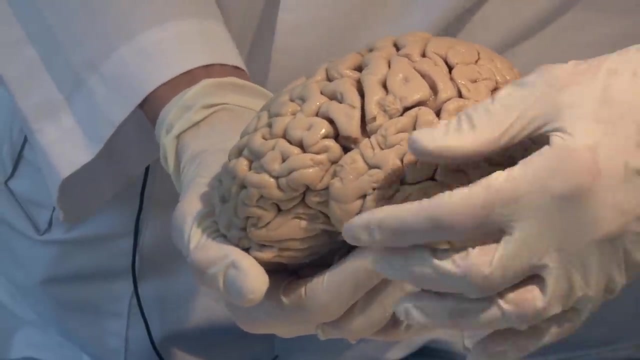 for visual computation and orientation and analysis. So we have our three lobes: occipital lobe, involved with vision, parietal lobe involved with sensation and integration of multiple modes of sensory input, and a frontal lobe with motor and higher order function. 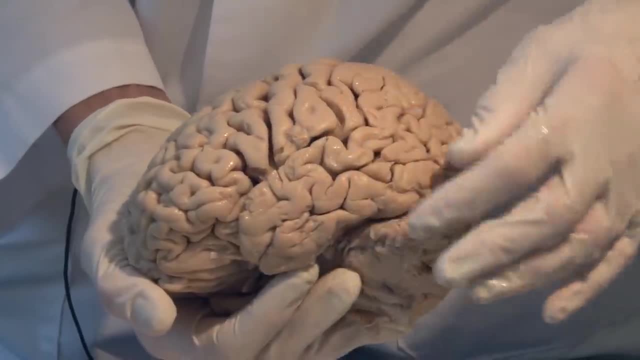 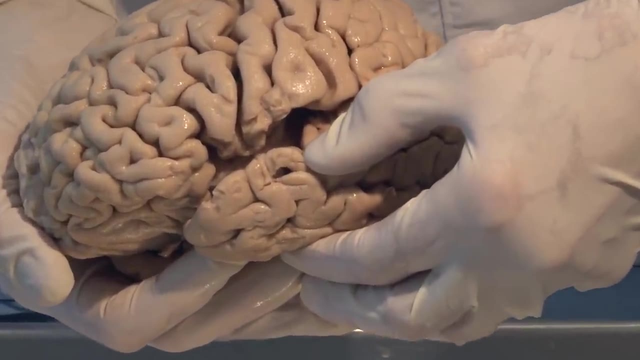 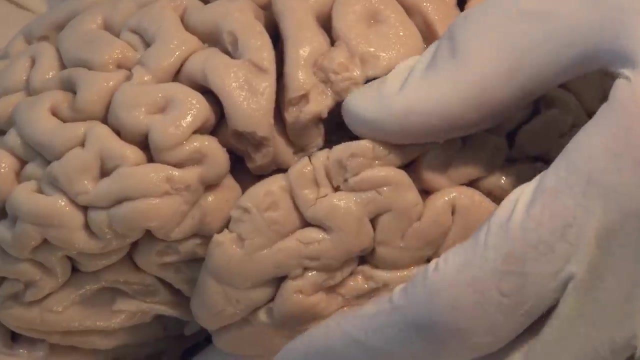 And this temporal lobe that is down here is very much involved with auditory information which is coming into this fissure here that I'm pulling down. This is the lateral fissure And auditory information- sound- comes to both hemispheres and is processed here. 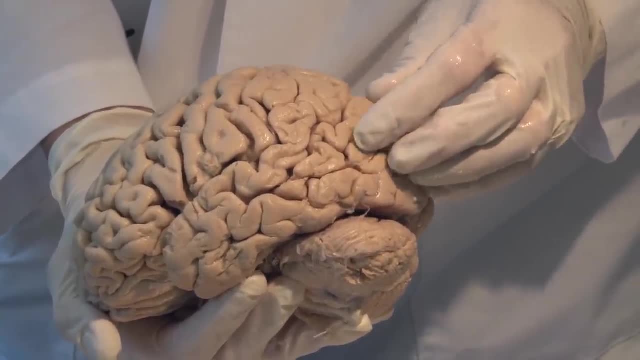 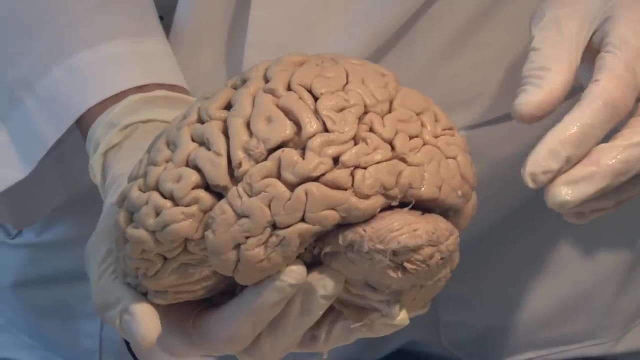 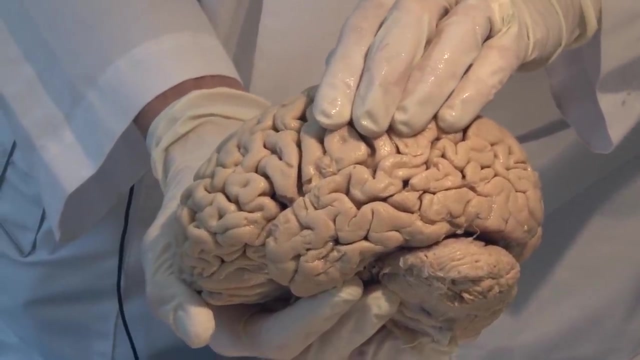 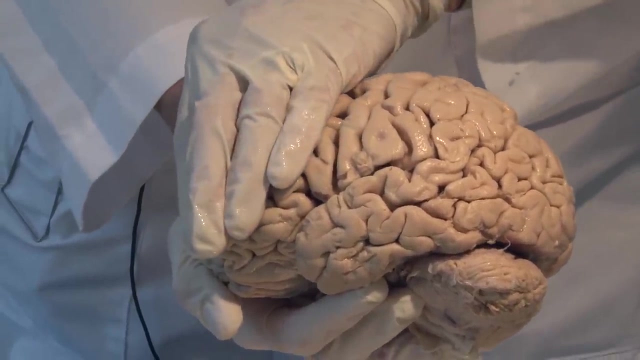 and we are very specialized as humans for visual computation and orientation and analysis. So we have our three lobes: occipital lobe, involved with vision, parietal lobe involved with sensation and integration of multiple modes of sensory input, and a frontal lobe with motor and higher order function. 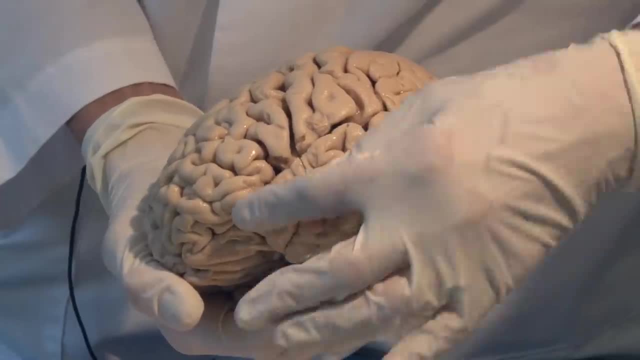 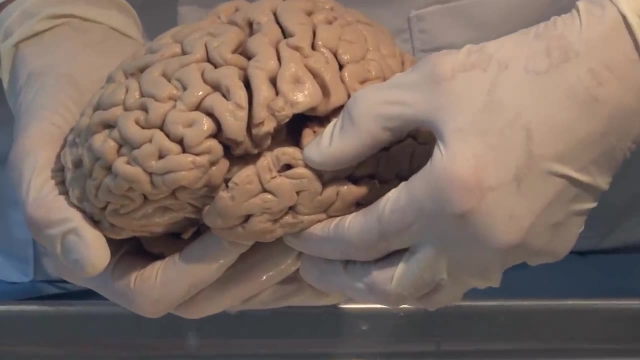 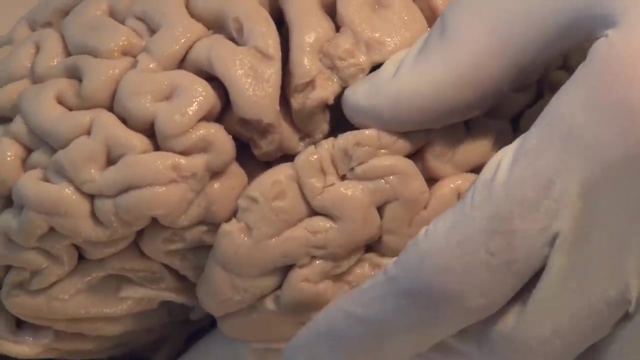 And this temporal lobe that is down here is very much involved with auditory information which is coming into this fissure here that I'm pulling down. This is the lateral fissure And auditory information- sound- comes to both hemispheres and is processed here. 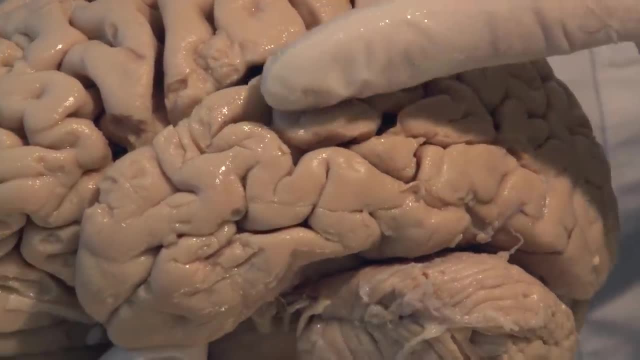 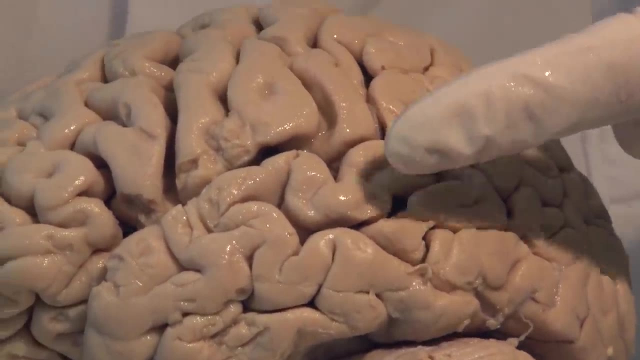 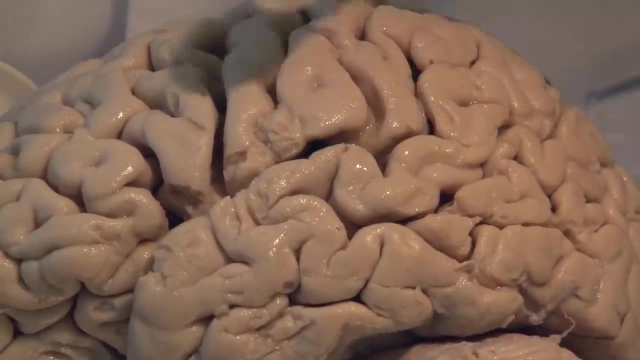 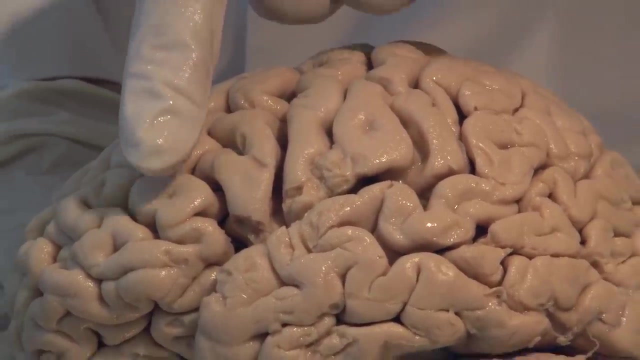 And this area behind me is the superior temporal gyrus. This back part here is involved in the comprehension of language. So you've got two language areas, an interpretive language area and a production language area. And when we study the consequences of cerebral stroke. 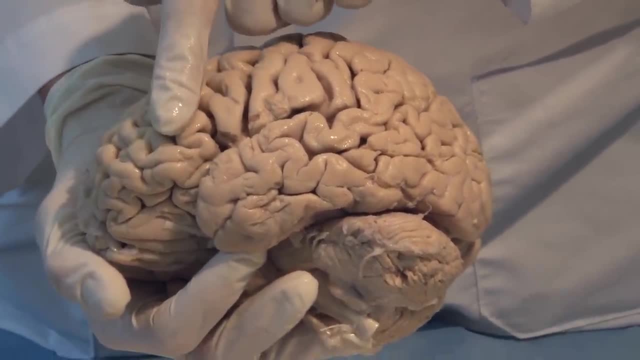 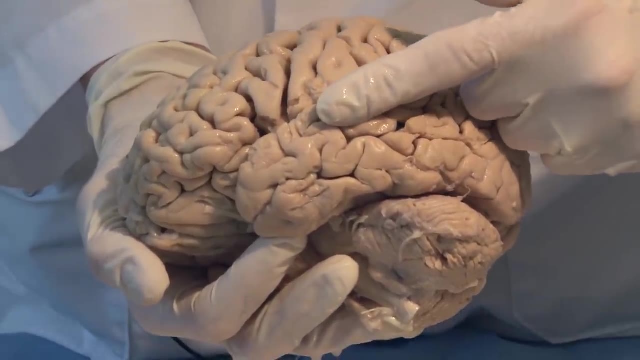 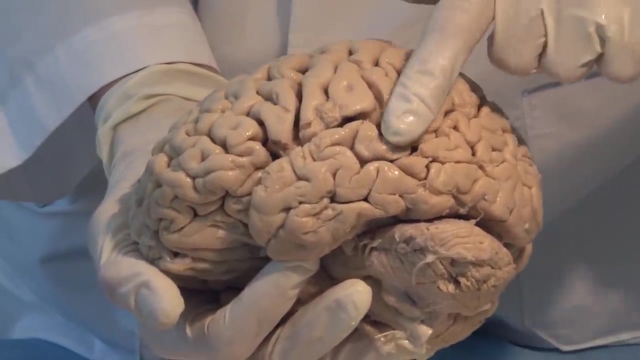 we'll see that some strokes can knock out one area and you'll have problems producing intelligible speech, while other areas leave you hearing perfectly fine but not understanding what you're hearing. And other lesions or damaging strokes that involve all of this area can leave you with a large deficit. 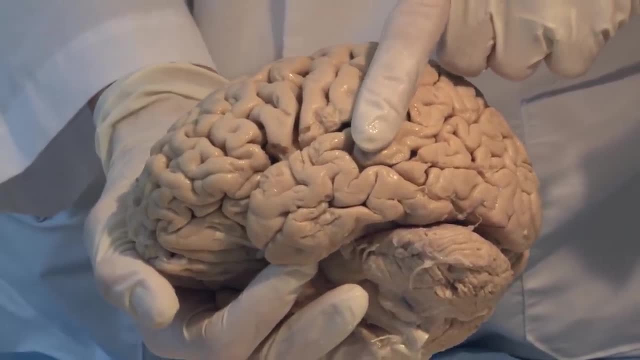 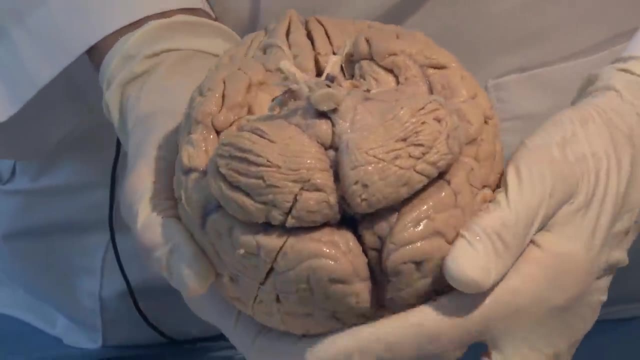 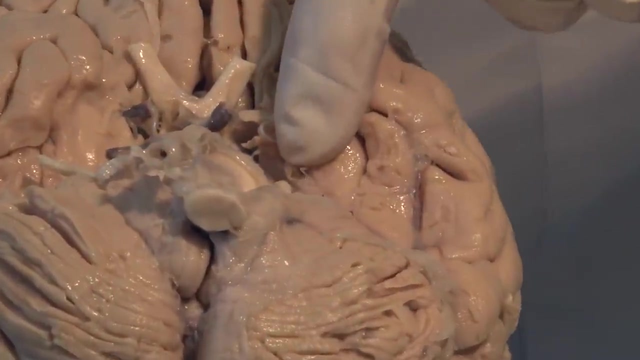 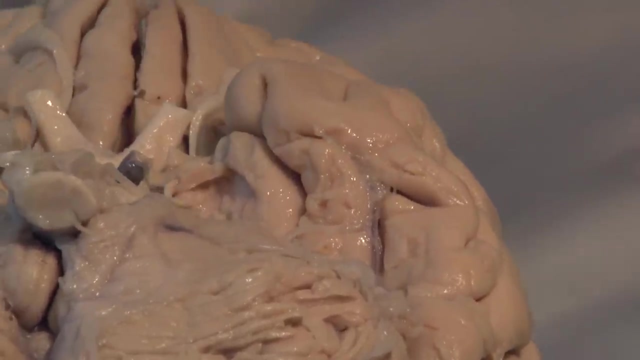 which we call global aphasia. Aphasia is a language disturbance. The temporal lobe, in addition to having an auditory function, has an area, underneath this gyrus here, which is required in one hemisphere for forming new memories. It's called the hippocampus. 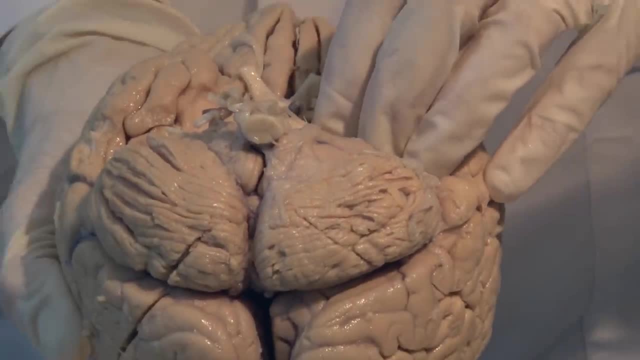 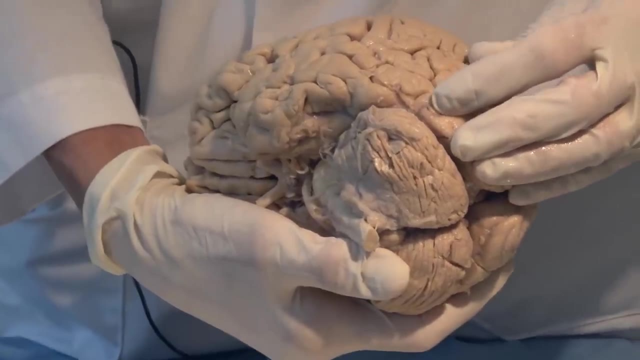 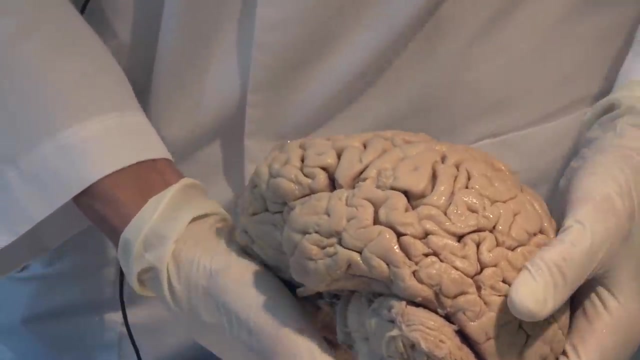 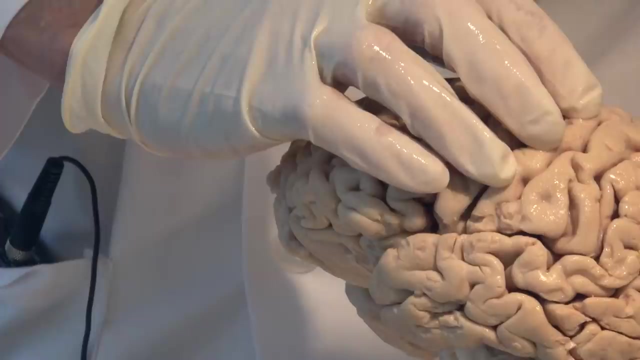 but it's not visible here. So temporal lobe- auditory and new memories. occipital lobe- visual information, processing and recognition. parietal lobe: somatic sensation from the face and the body. frontal lobe- motor execution voluntarily. 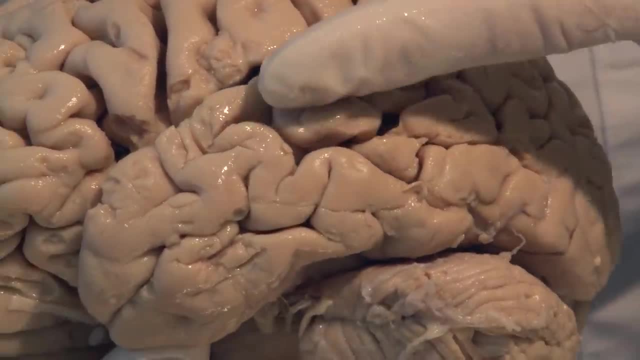 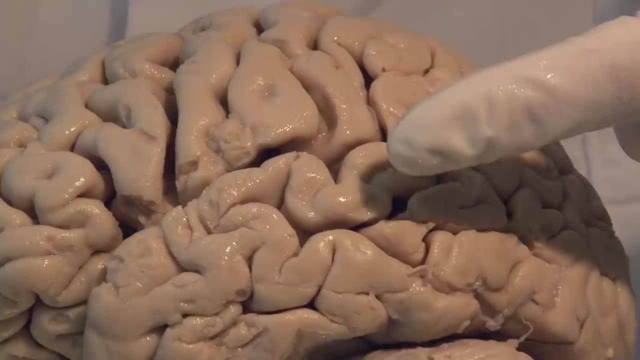 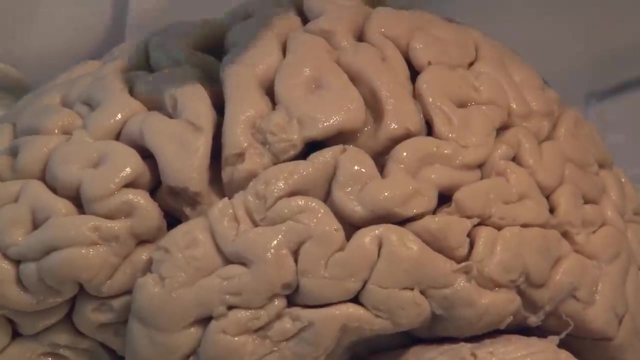 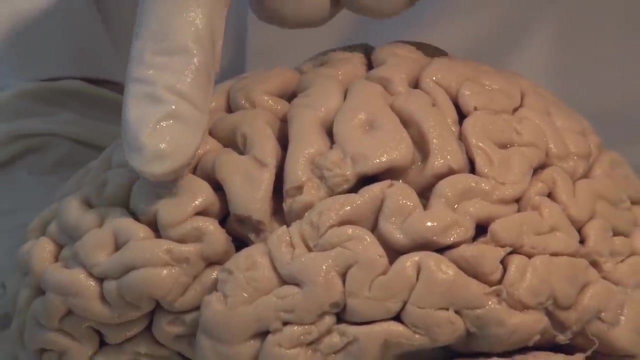 And this area behind it, the superior temporal gyrus. this back part here is involved in the comprehension of language. So you've got two language areas: an interpretive language area and a production language area. And when we study the consequences of cerebral stroke, 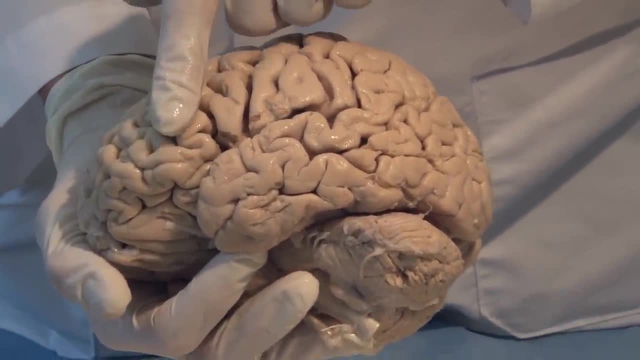 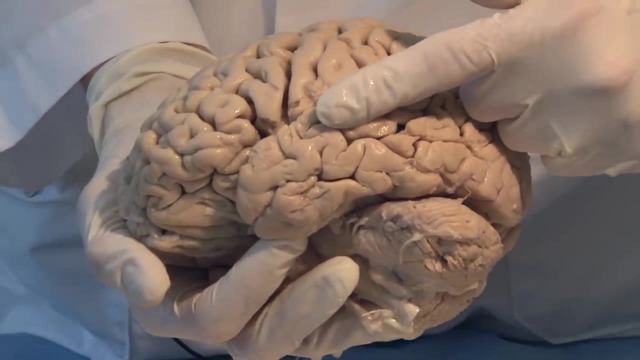 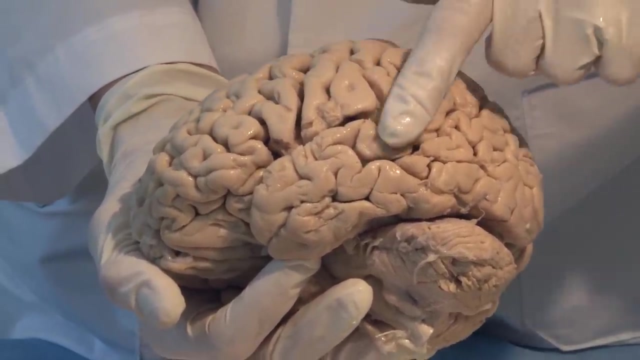 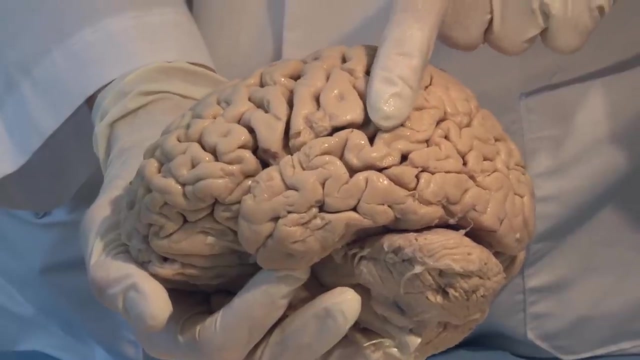 we'll see that some strokes can knock out one and you'll have problems producing intelligible speech, while other areas leave you hearing perfectly fine but not understanding what you're hearing. And other lesions or damaging strokes that involve all of this area can leave you with a large deficit, which we call global aphasia. 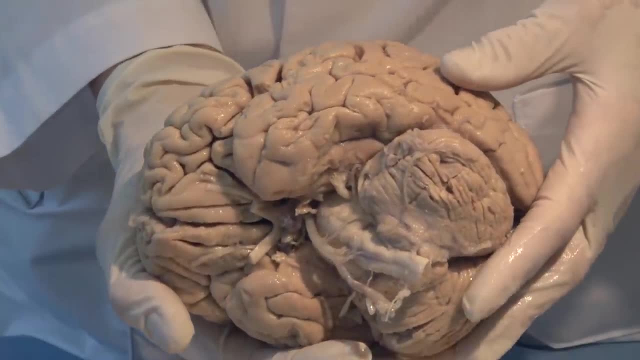 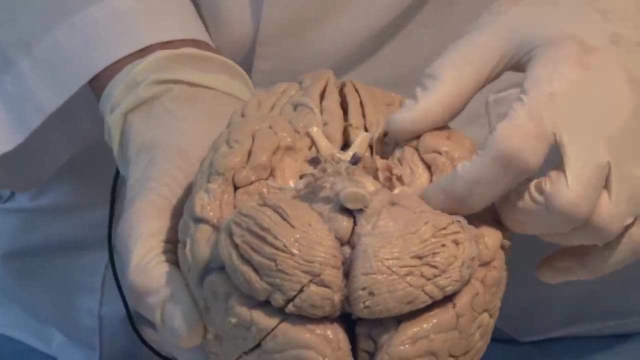 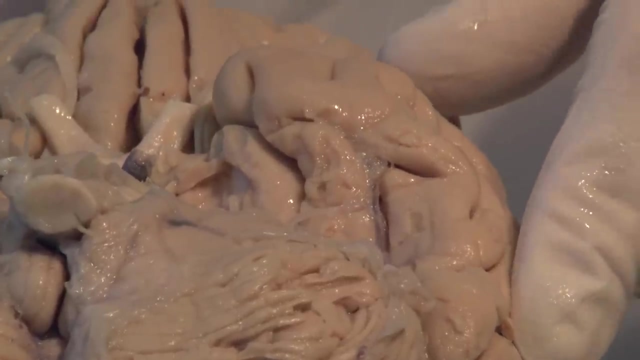 Aphasia is a language disturbance. The temporal lobe, in addition to having an auditory function, has an area underneath this gyrus here, which is required in one hemisphere for forming new memories. It's called the hippocampus, but it's not visible here. 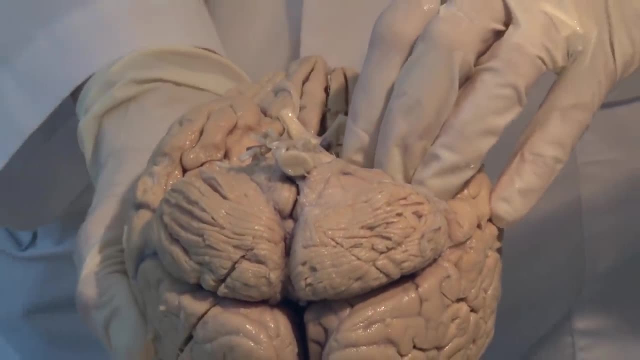 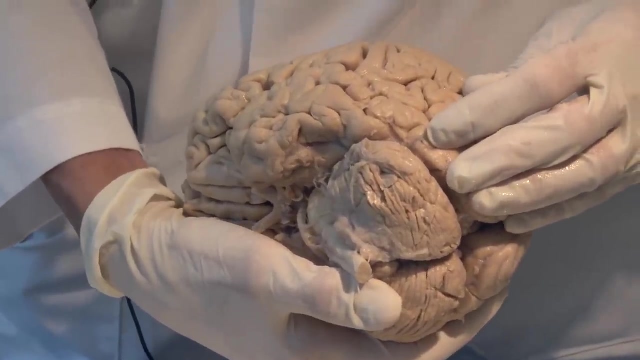 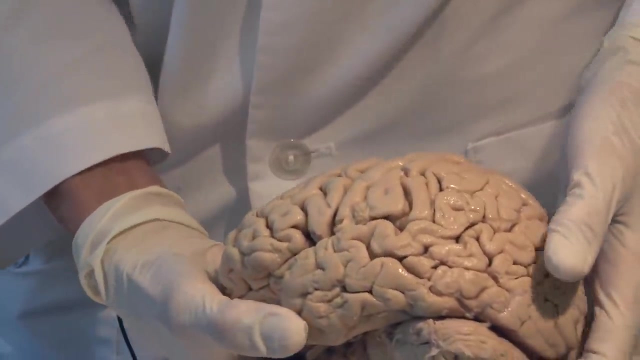 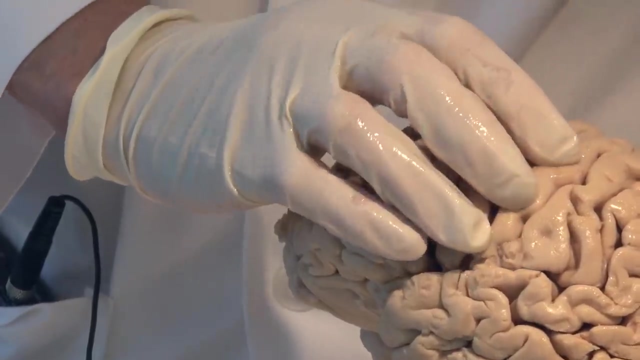 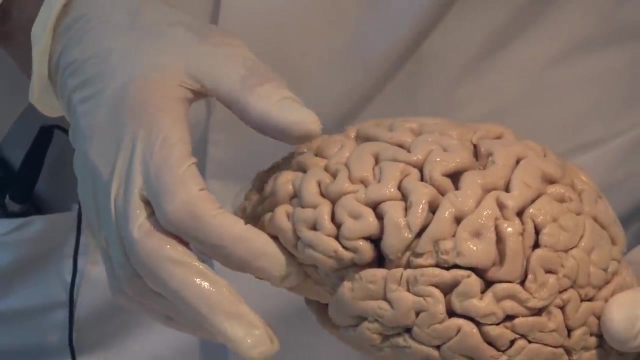 So: temporal lobe, auditory and new memories. occipital lobe, visual information processing and recognition. parietal lobe, somatic sensation from the face and the body. frontal lobe, motor execution, voluntarily planning and execution of appropriate judgment and actions. 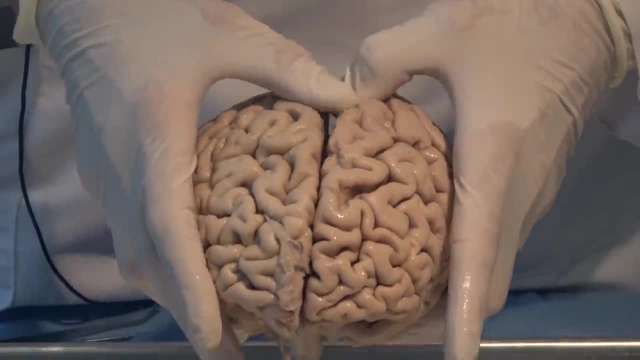 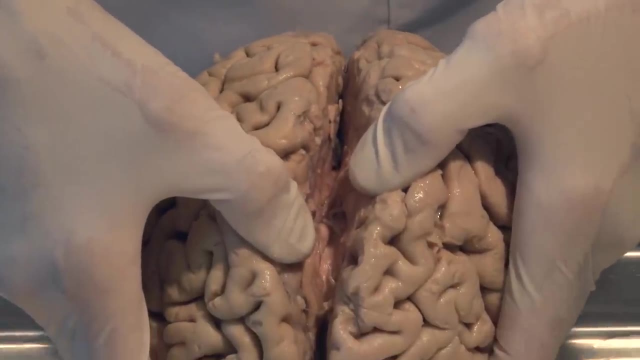 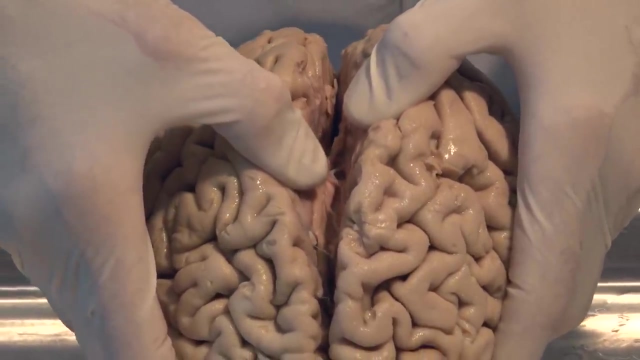 The two hemispheres are not identical, and later we'll talk about special localizations between the hemispheres, But right now I just want to point to the fact that the two hemispheres are held together by a large band of fibers called the corpus callosum. 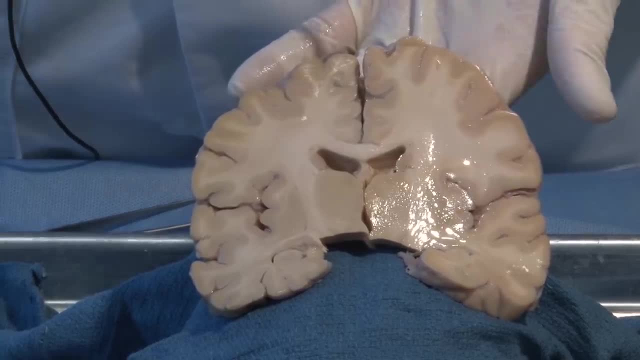 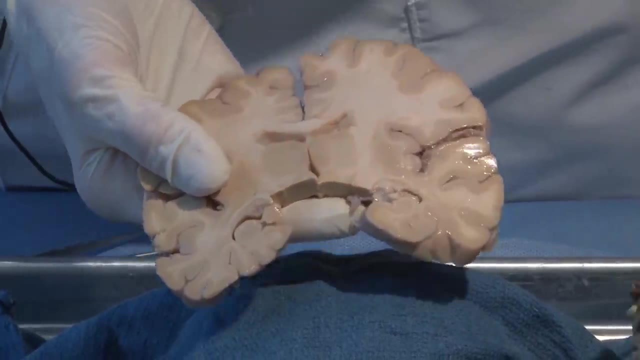 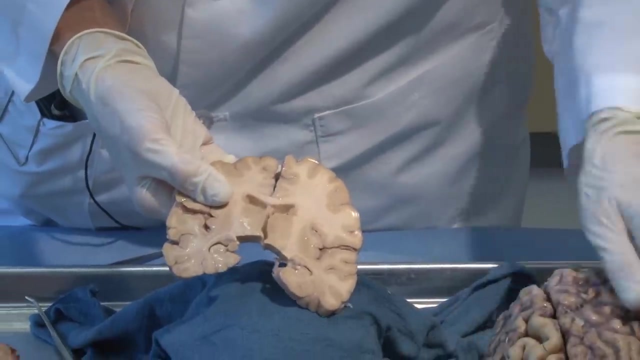 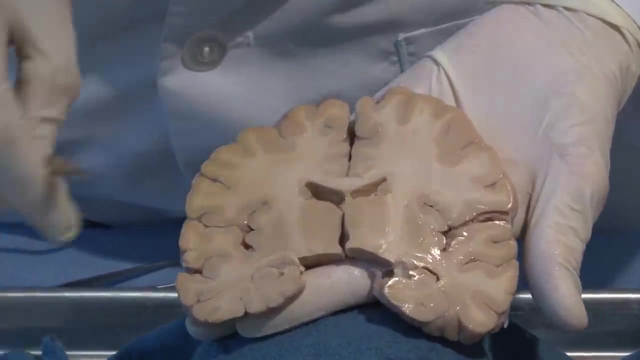 What I have here is a coronal section through the brain. What we've done is we've taken our brain and we've sliced it like through this way, and so this is called a coronal or frontal section, And I'm going to rest it here so that you can see. 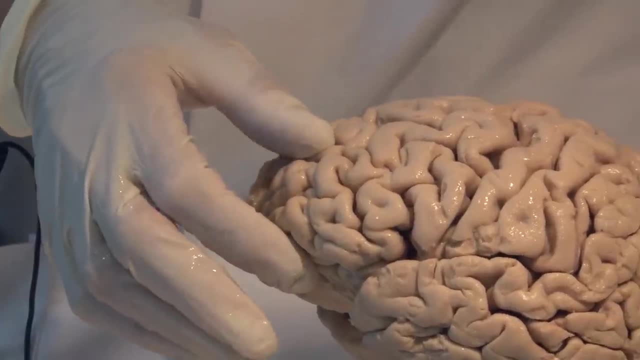 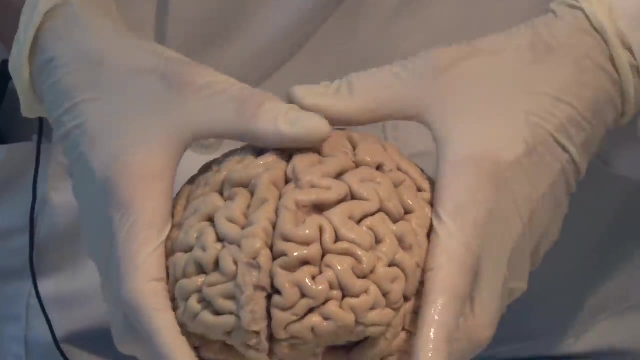 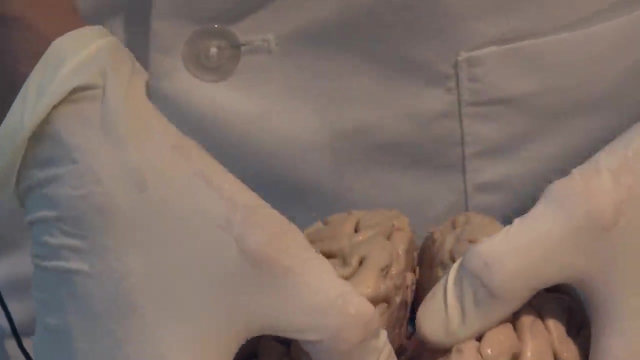 planning and execution of appropriate judgment and actions. The two hemispheres are not identical, and later we'll talk about special localizations between the hemispheres, but right now I just want to point to the fact that the two hemispheres are held together. 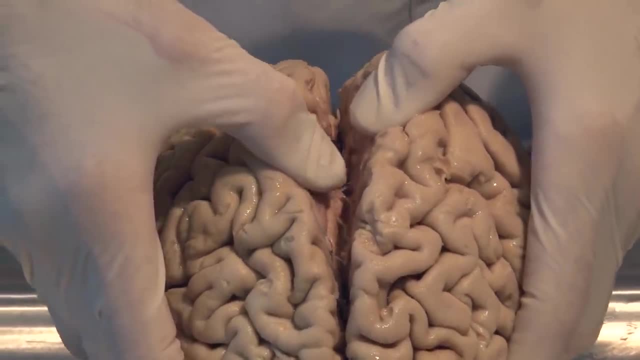 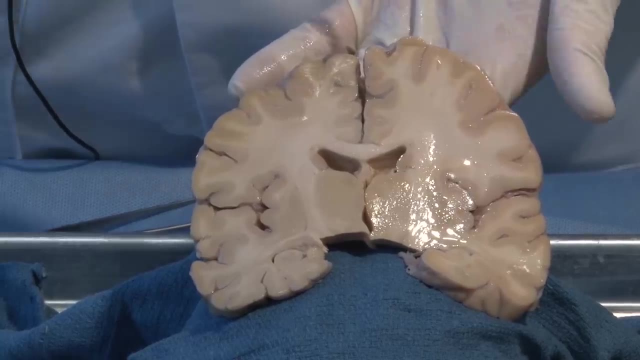 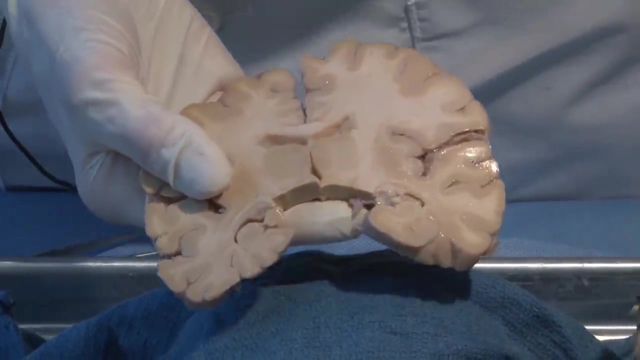 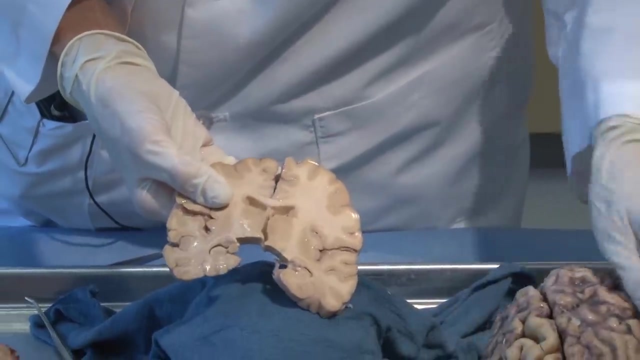 by a large band of fibers called the corpus callosum. What I have here is a coronal section through the brain. What we've done is we've taken our brain and we've sliced it like through this way, and so this is called a coronal or frontal section. 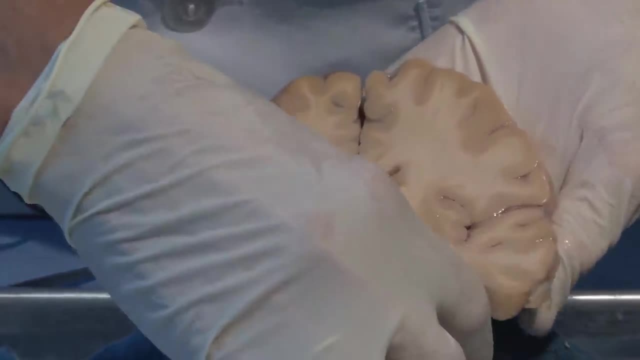 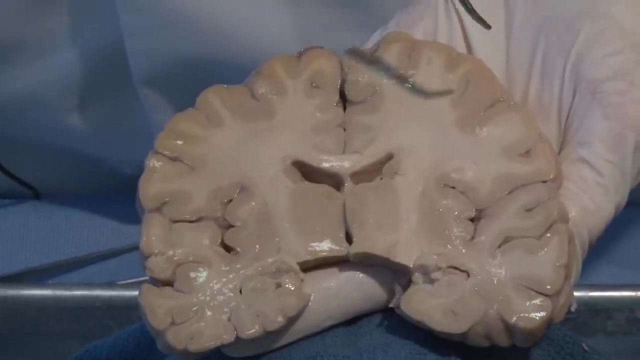 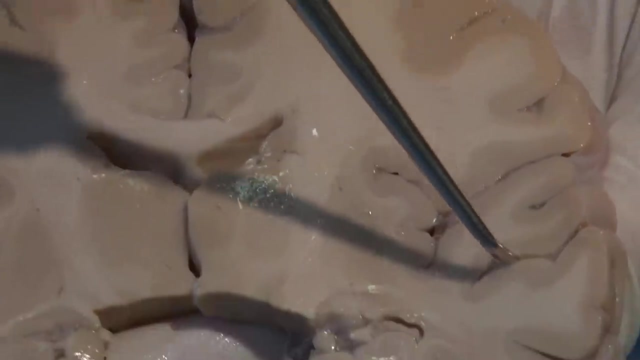 And I'm going to rest it here so that you can see the internal structure of the brain. We'll deal with these in more detail, but right now you can see that those gyri that we were looking at and the sulci, the dips in between, 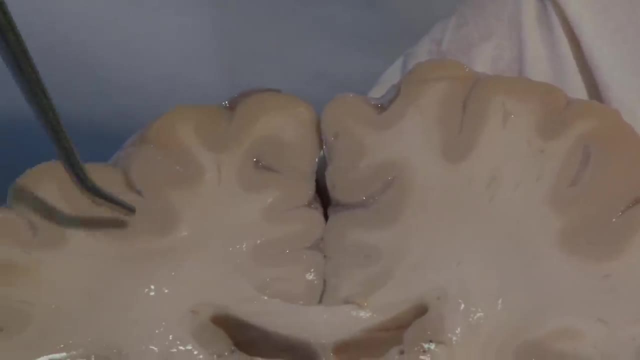 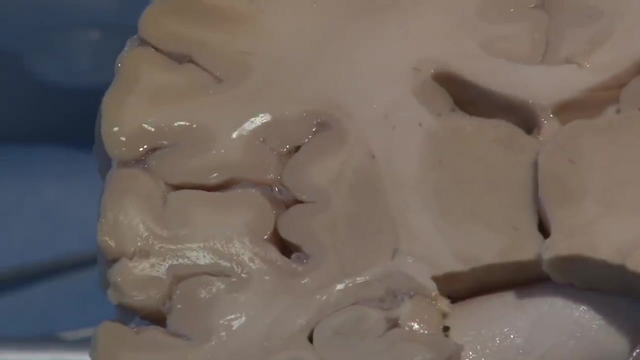 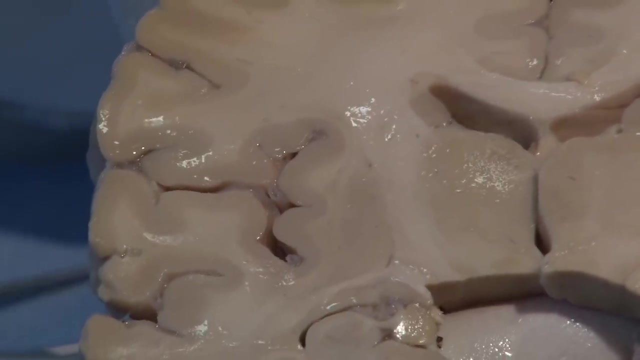 can be easily distinguished And the gyri are covered with a nice layer beige in color, and that is your gray matter, as we say, of the cerebral cortex- Maybe we should have called it beige matter- And beneath it is a lighter area. 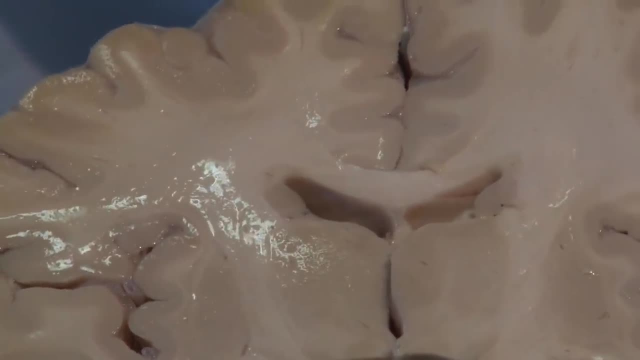 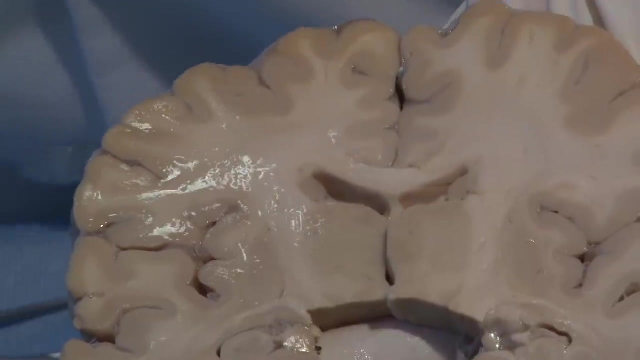 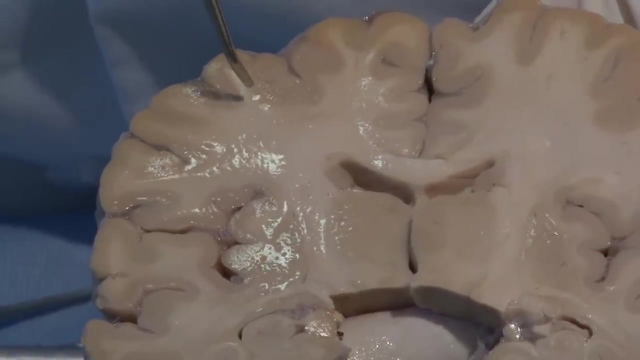 which we call the white matter. In general, gray matter consists of cell bodies, both neurons and glia, and white matter are axons. Axons are the processes of neurons either coming to the cerebral cortex or leaving the cerebral cortex and descending to lower brain structures. 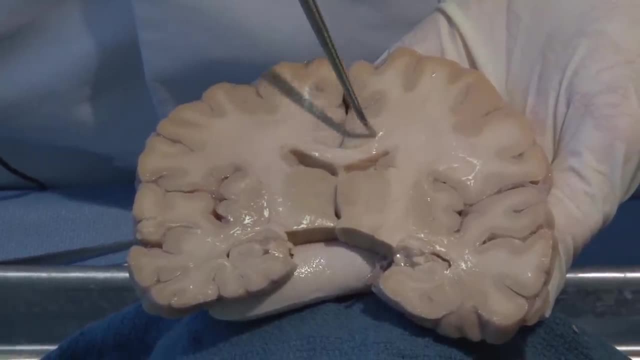 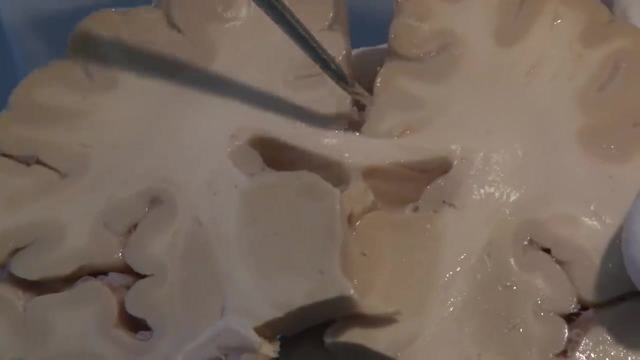 An example of white matter here is this band of fibers called the corpus callosum. It was that band that held the two hemispheres together When we were looking down through that inner hemispheric fissure. the base of that was this band of white matter. 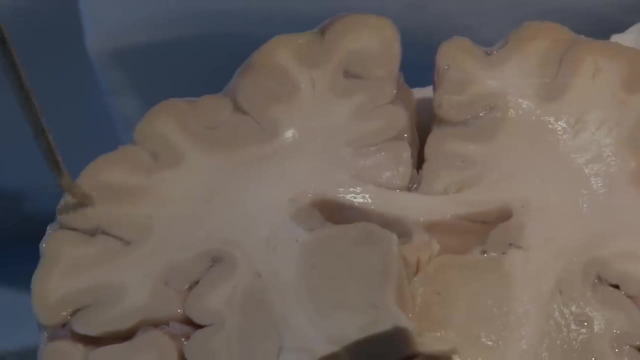 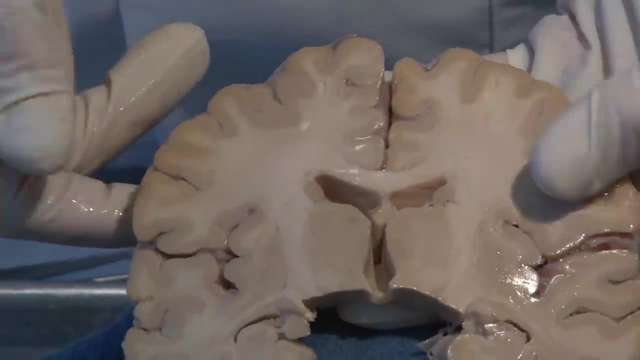 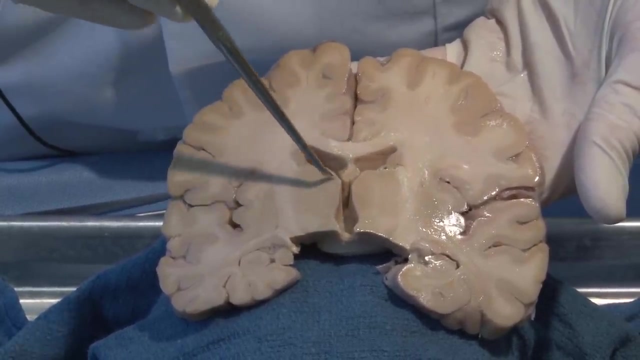 connecting similar areas or homotopic areas of one hemisphere with the other, And this is a way that the right and the left hemispheres can communicate. In addition, they can communicate through structures like this deep area. You notice, it's beige. 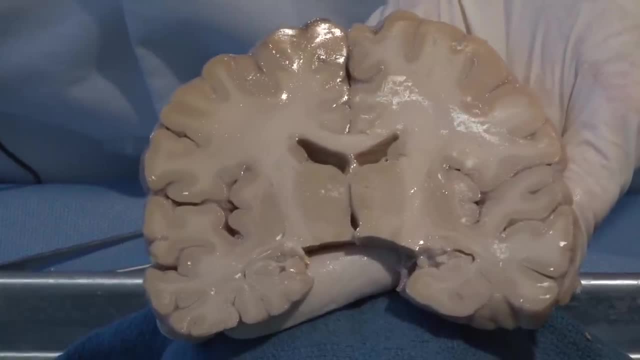 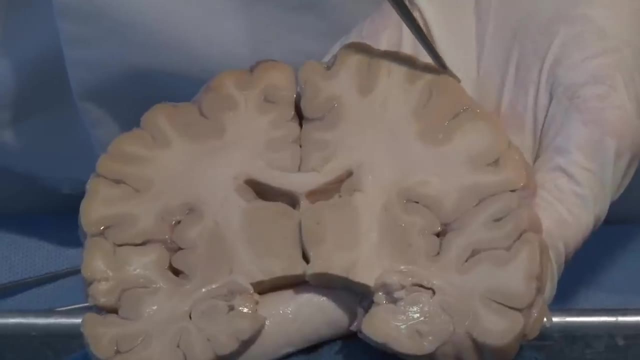 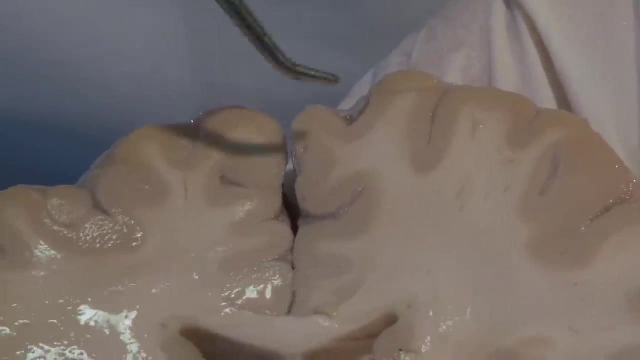 the internal structure of the brain. We'll deal with these in more detail, but right now you can see that those gyri that we were looking at and the sulci, the dips in between, can be easily distinguished And the gyri are the parts of the brain. 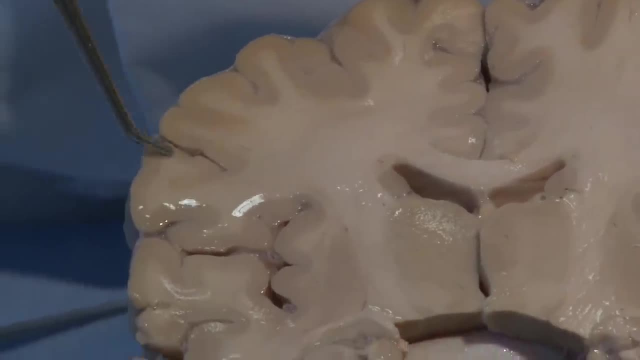 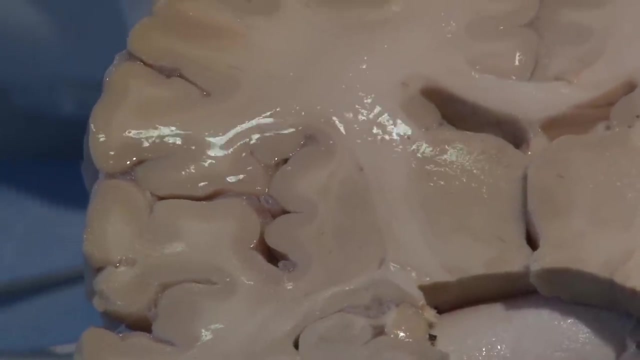 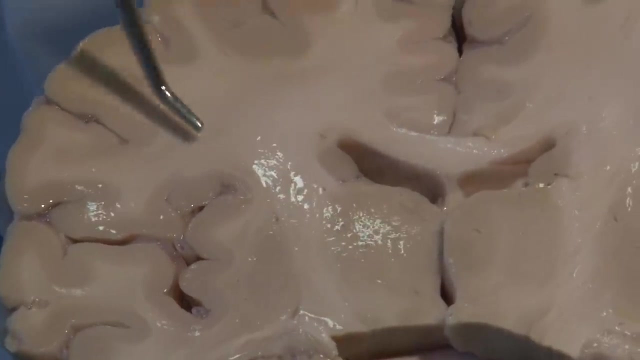 that are covered with a nice layer beige in color, and that is your gray matter, as we say, of the cerebral cortex. Maybe we should have called it beige matter, And beneath it is a lighter area which we call the white matter. 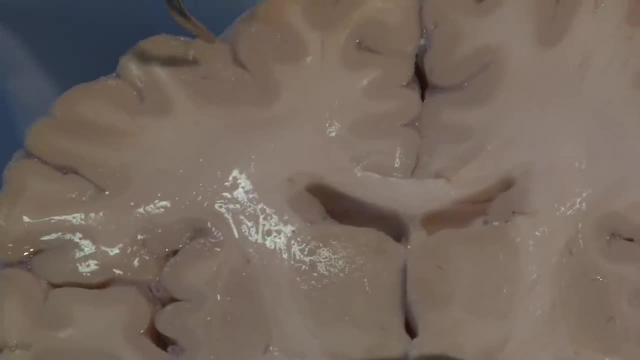 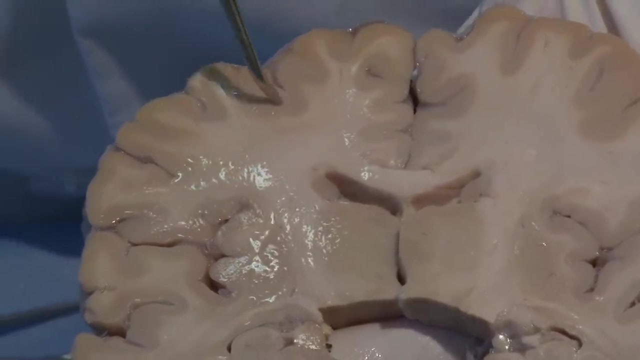 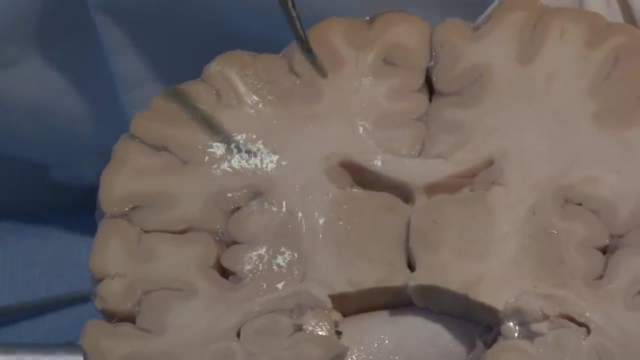 In general, gray matter consists of cell bodies, both neurons and glia, and white matter are axons. Axons are the processes that connect the two neurons, either coming to the cerebral cortex or leaving the cerebral cortex and descending to lower brain structures. 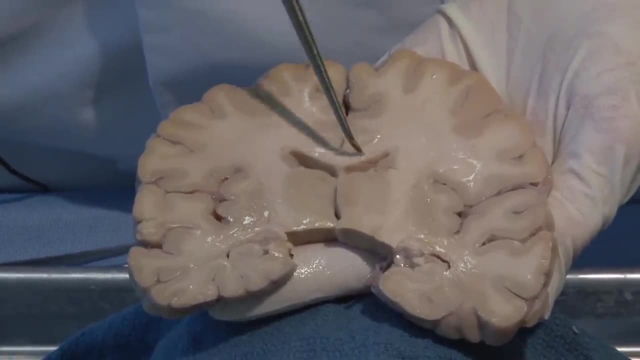 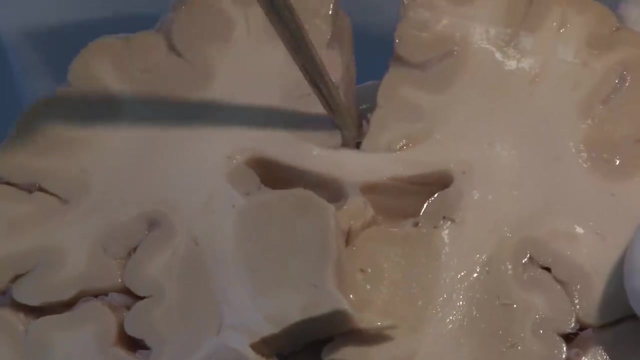 An example of white matter here is this band of fibers called the corpus callosum. It was that band that held the two hemispheres together When we were looking down through that inner hemispheric fissure. the base of that was this band of white matter. 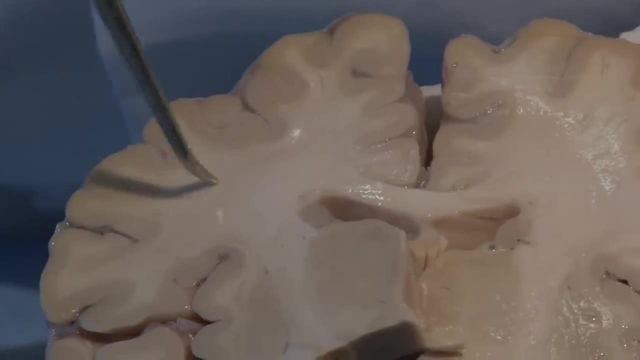 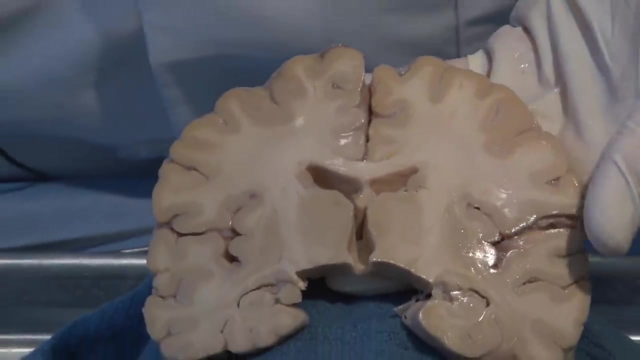 which was the corpus callosum, And the corpus callosum was the one that was connecting the two hemispheres and connecting the two hemispheres together. So we were connecting similar areas, or homotopic areas of one hemisphere with the other. 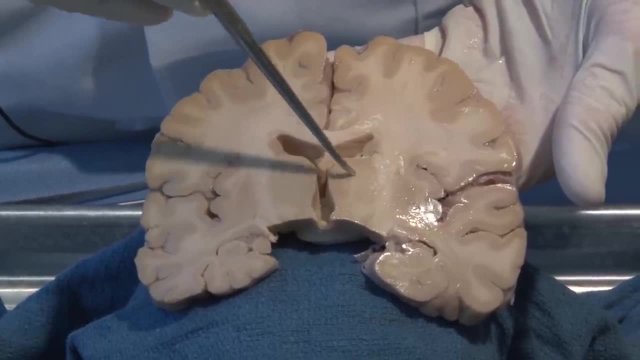 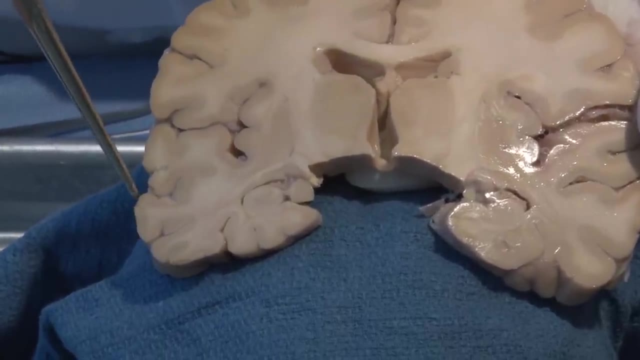 And this is a way that the right and the left hemispheres can communicate. In addition, they can communicate through structures like this deep area. You notice it's beige, so it's mainly cell bodies, And you can see here if I prop this up. 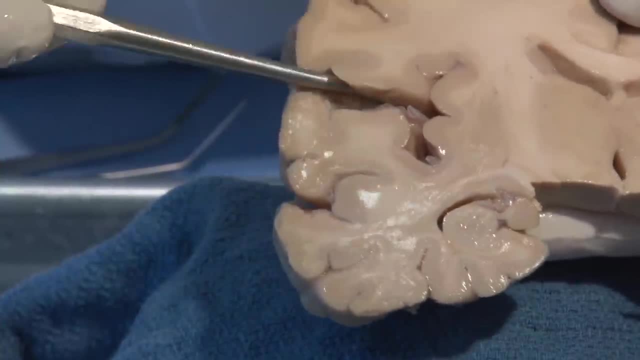 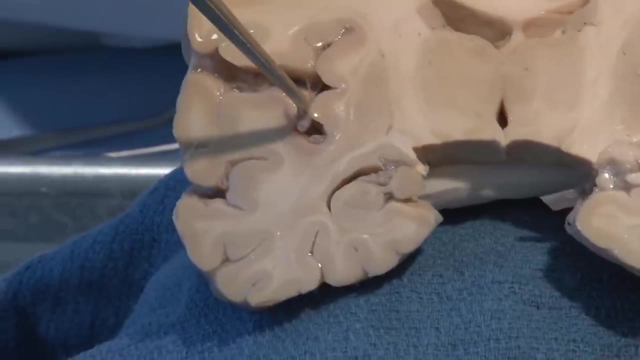 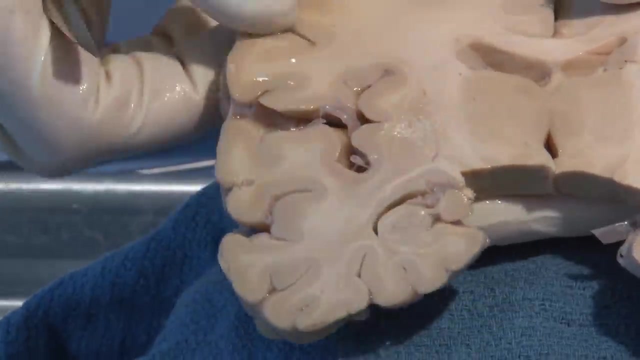 and pull it down a little bit, you can see that large lateral fissure that we saw on the lateral surface. That means that this is the temporal lobe. You can even see a blood vessel in there, This bit of cortex buried underneath the hemispheric temporal and parietal lobes. 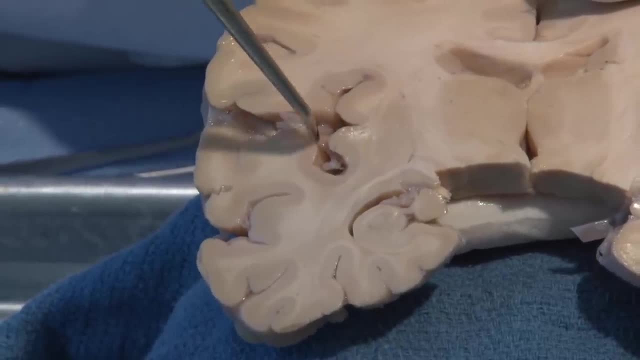 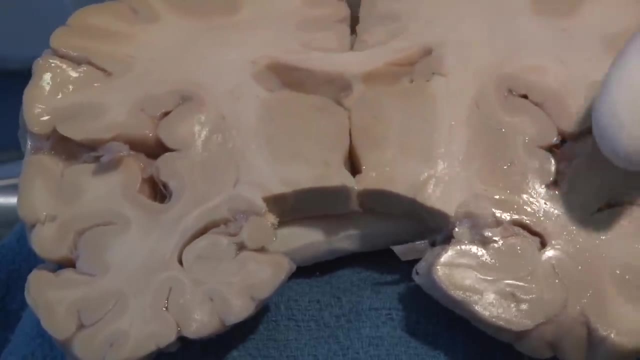 is the insula. We're not going to deal with that, but it does have a name. It's where the cortex got buried and became more and more convoluted. This is parietal or it could be motor cortex- I can't tell- with an isolated section exactly. 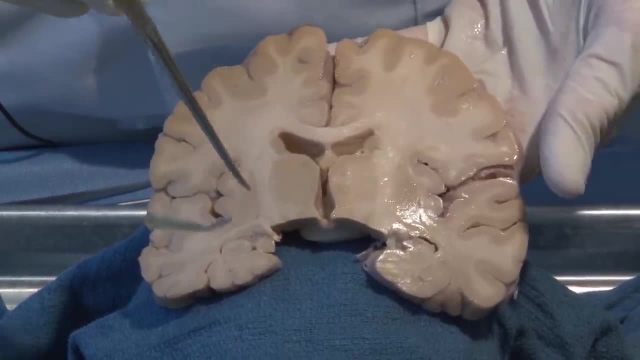 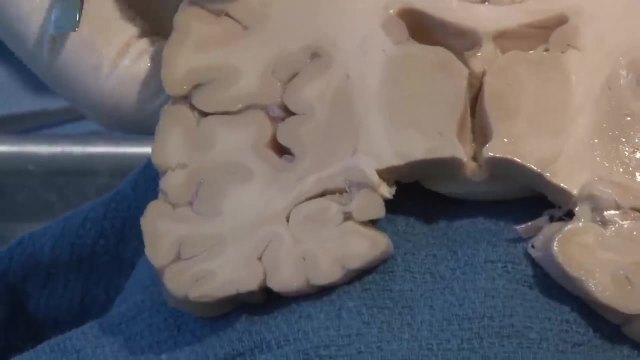 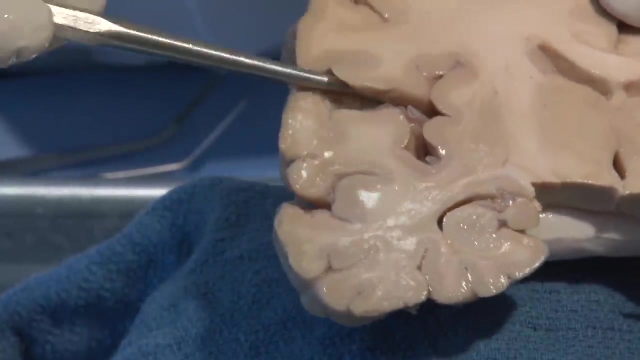 so it's mainly cell bodies, a deep structure called the thalamus, And here we can see the temporal lobe that we were looking at on the surface. Notice here: if I prop this up and pull it down a little bit, you can see that large lateral fissure. 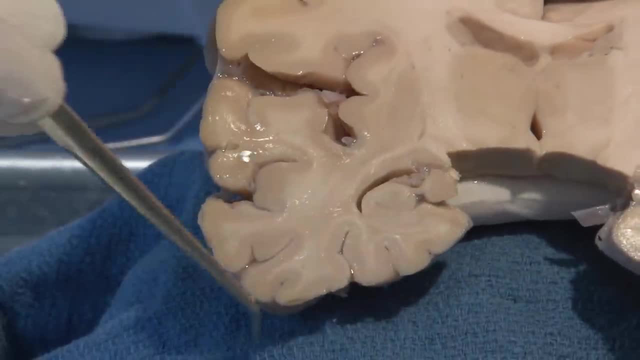 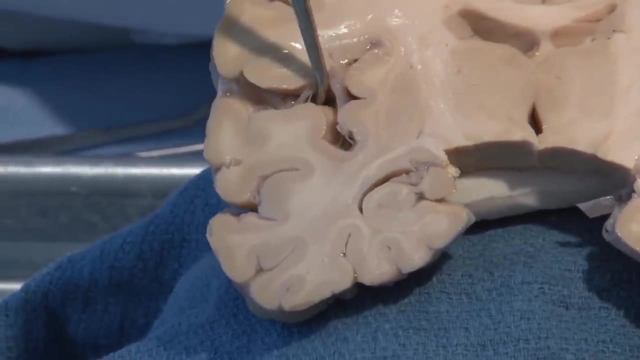 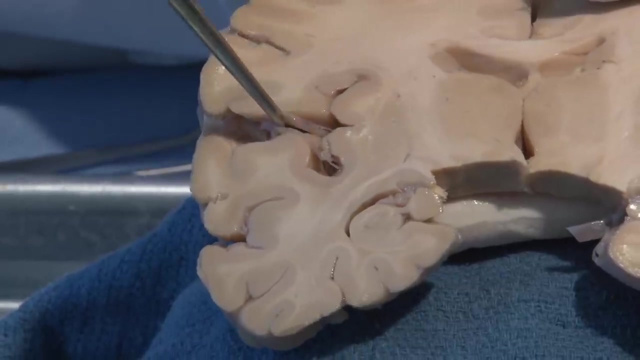 that we saw on the lateral surface. That means that this is the temporal lobe. You can even see a blood vessel in there. This bit of cortex buried underneath the hemispheric, temporal and parietal lobes is the insula. We're not going to deal with that. 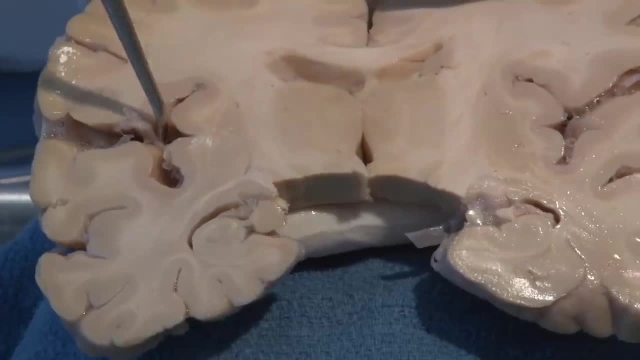 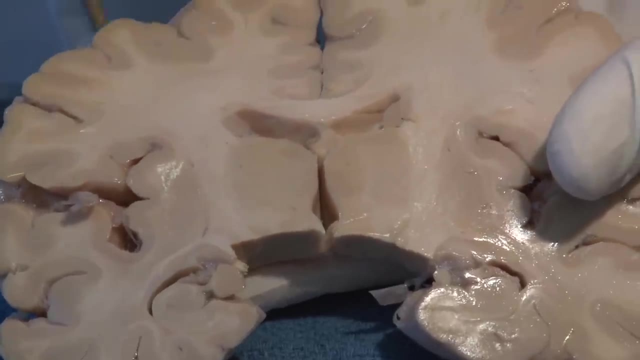 but it does have a name. It's where the cortex got buried as it became more and more convoluted. This is parietal or it could be motor cortex. I can't tell with an isolated section exactly if they're in the frontal lobe or the parietal lobe. 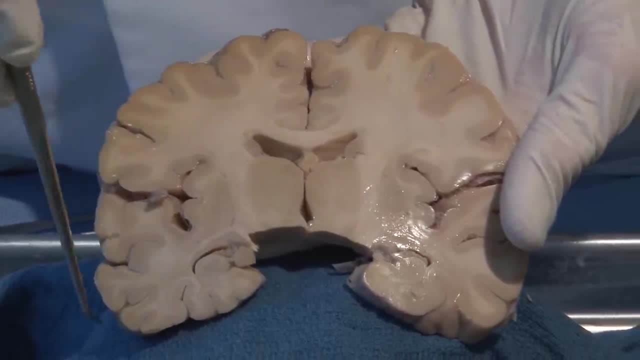 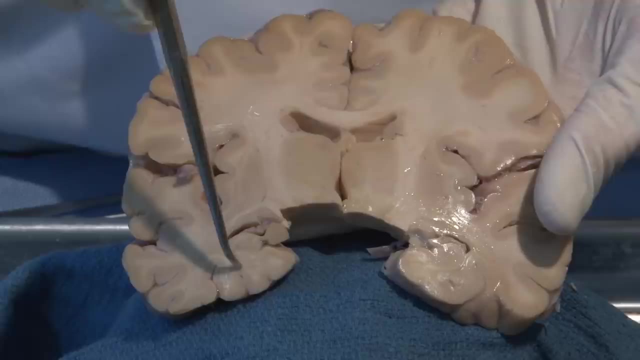 It doesn't really matter- And remember I told you that one of the functions of the temporal lobe, in addition to the auditory region, was an area involved in memory. That area is called the hippocampus and it's curled up here right in this medial part. 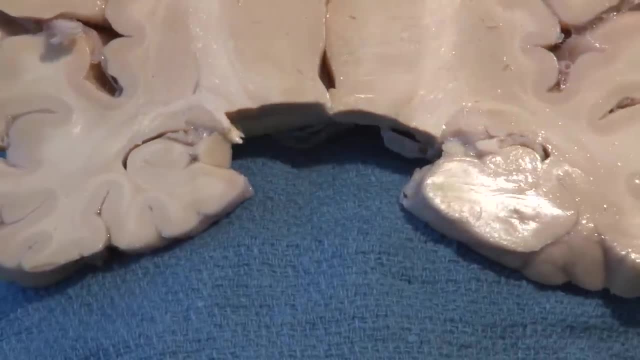 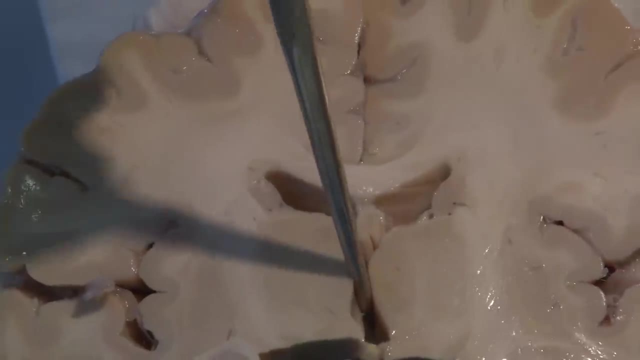 of the temporal lobe. The other major structure you see in a cross-section like this or a coronal section, are these holes in the brain? One here, one here, one here, a little bitty one here and here. 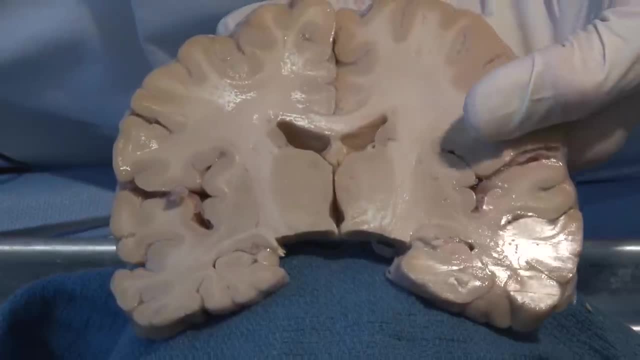 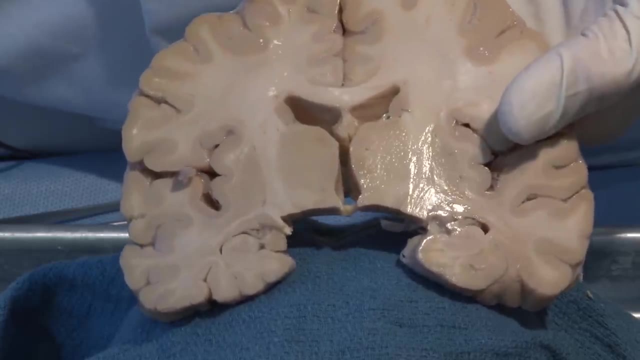 These form part of the ventricle system, which we will explore further, But right now just know that they're filled with cerebral spinal fluid And the leptomeninges, or the pia, and the arachnid on the surface. 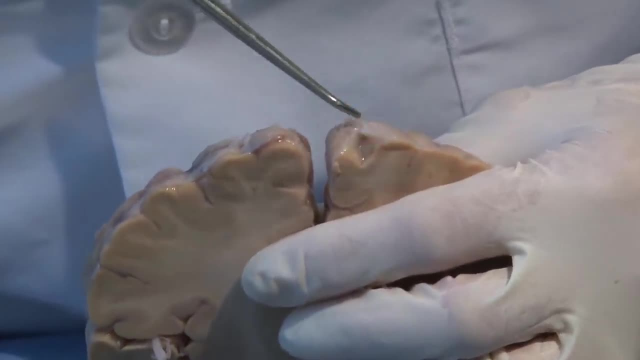 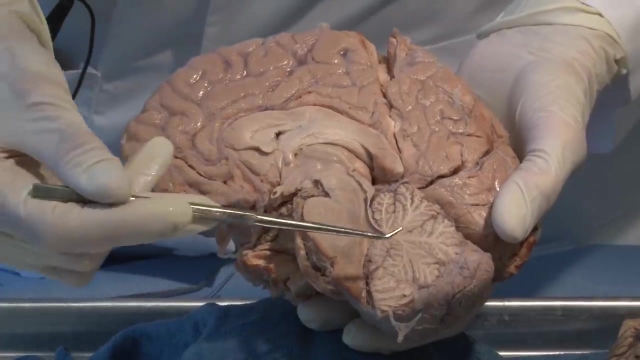 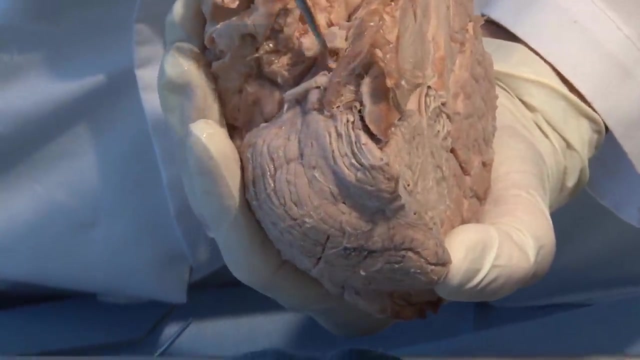 if we can zoom in a little bit, we can see them delicately covering the surface of the brain. The main thing I want you to see on this brain is the brain stem. So this is the cerebellum that we saw before, up to the side. 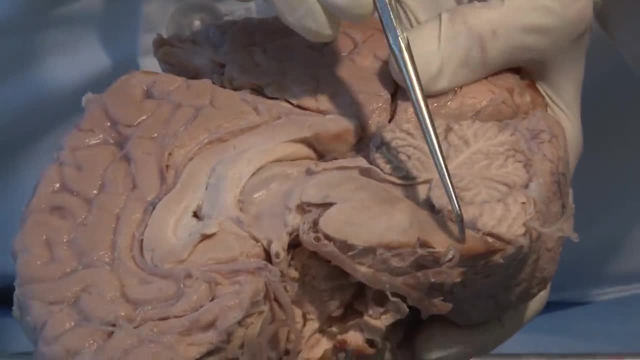 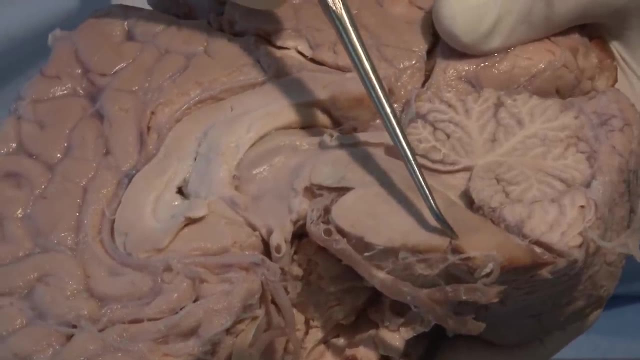 and the brain stem recall, was in the middle. Here we have the brain stem on a mid-sagittal. This is cut in the middle, So this is a mid-sagittal section. Here's a bit of the medulla. 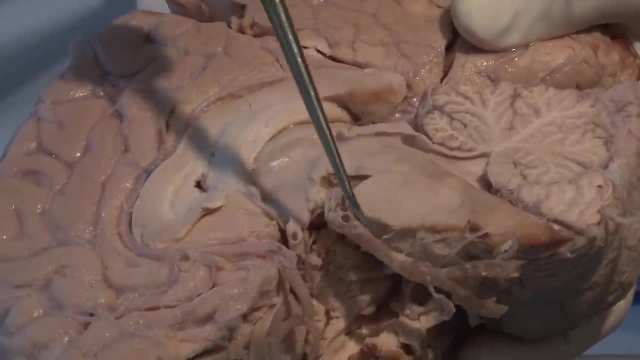 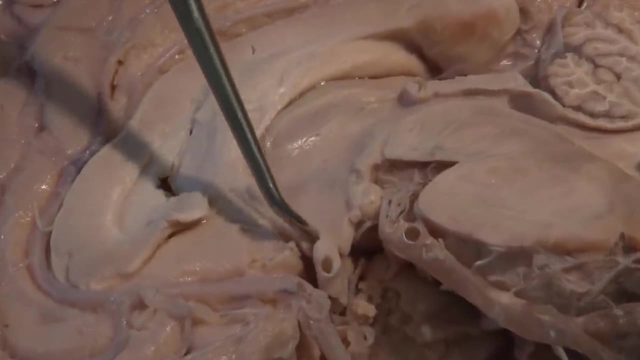 Here is the pons, with a big basilar artery creeping up over it, And here is the midbrain, often hard to see, And finally then we have deep structures such as the thalamus, And we can see many of the vessels. 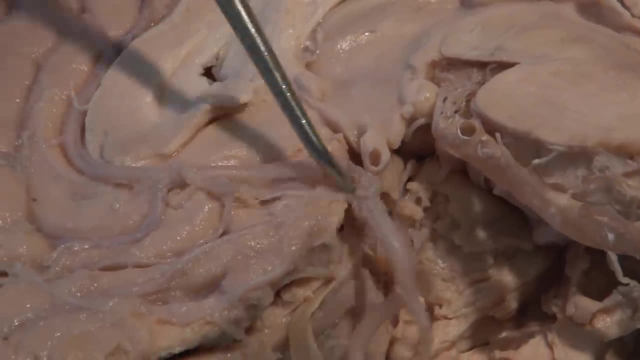 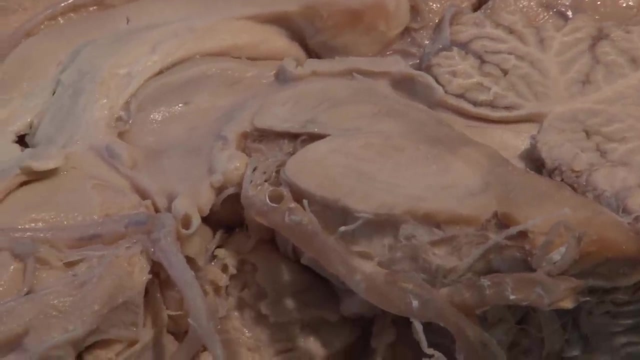 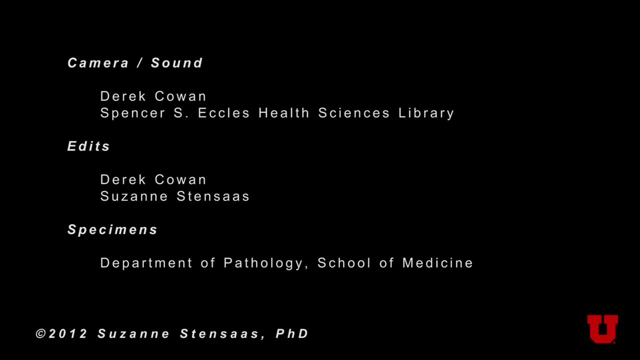 like the anterior cerebral artery here, as well as spaces such as the ventricular system, which we'll look at in more detail. So now we're in the middle. This is basically a big, big, big piece of the brain. So this is the brain. 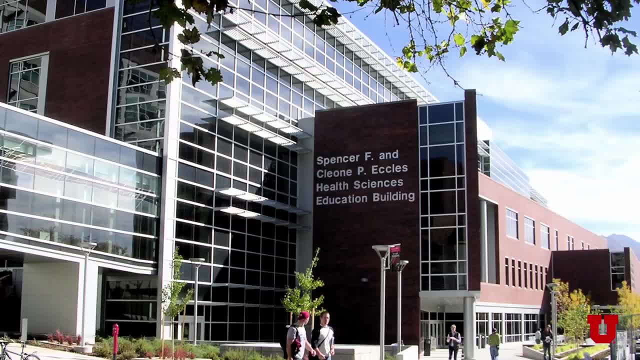 This is the mitral valve which we're in. This is the amyloid valve, the perioc Gong and this is the diaphragm of the amyloid valve. These are what we call the scapula And this is where the metastatic nervous system works, which is the middle, and here the cortex is located, And what you see here is the salivary gland. So you can notice a couple of things. I'll give you a pause here. The salivary gland is two places in the brain. 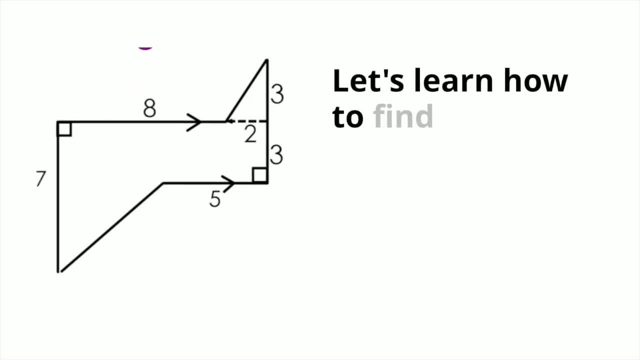 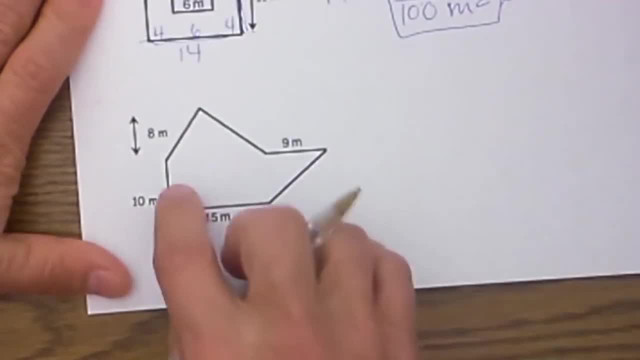 I wanted to do one that had three parts. This one has three sections and you could use the method where you fill the whole area in and then subtract parts, but you would have one, two, three parts. I think this one is just as easy to divide up into sections. I wanted 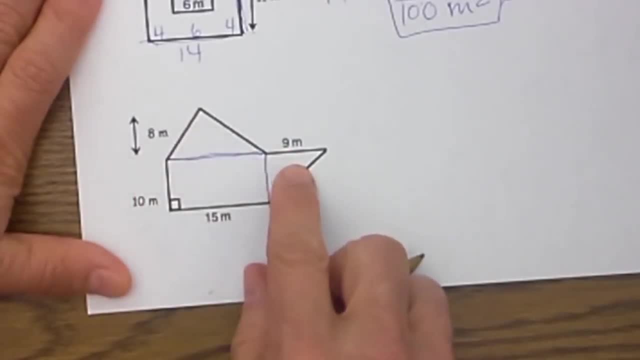 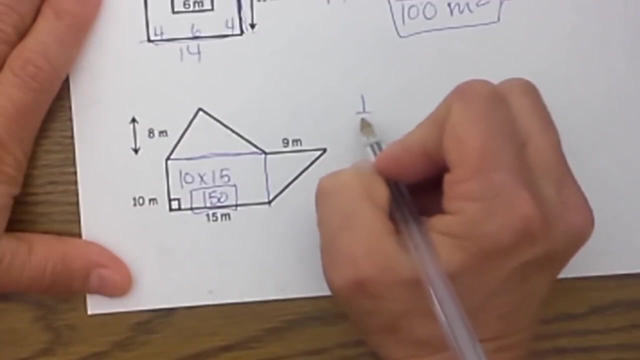 to do one with a triangle. This one has two triangles. Let's see if we can figure this one out. The area of the rectangle is just 10 times 15, which is 150 square meters. Remember, the area of a triangle is one half the base times the height. We need to know the base. 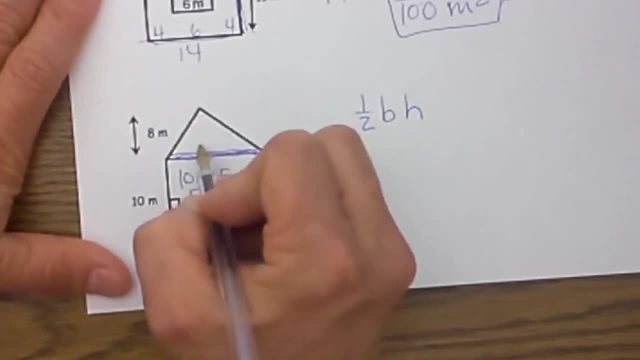 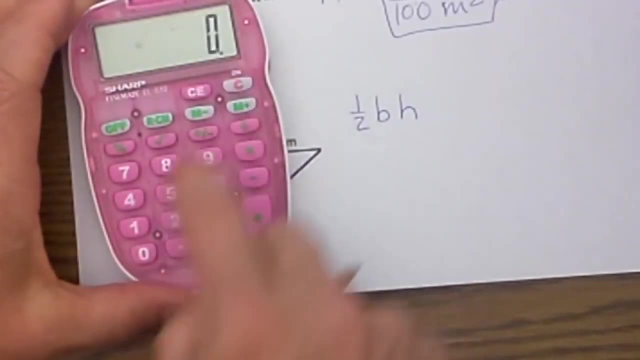 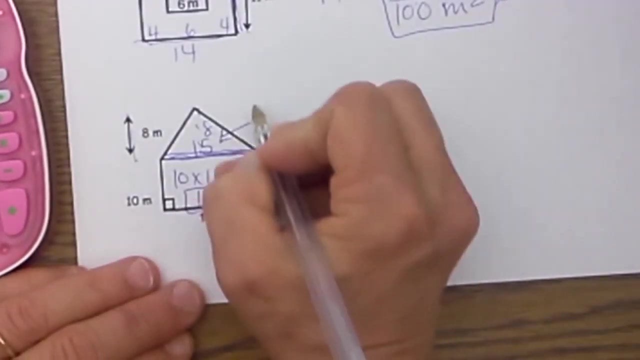 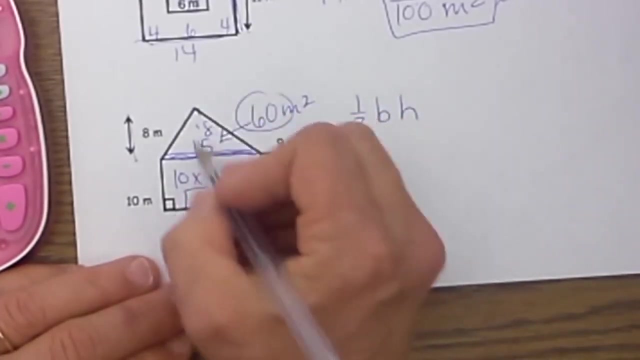 of this triangle, which we do because it is parallel to this piece. The height inside here is 8.. Let's multiply that out. We have 15 times 8, and then we divide that by 2. to multiply by half, That section is 60 square meters. So we have 150 for the bottom and 60 for this.